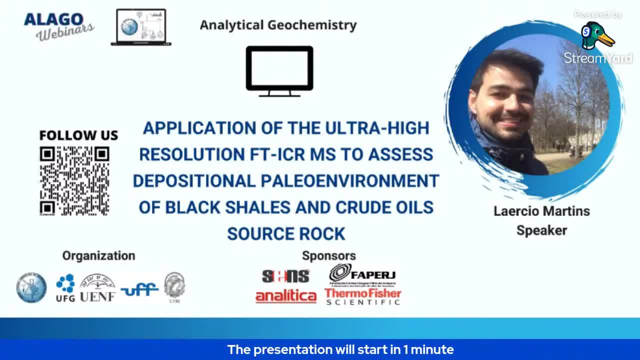 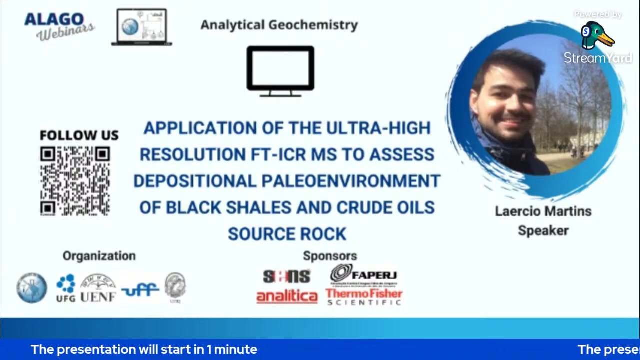 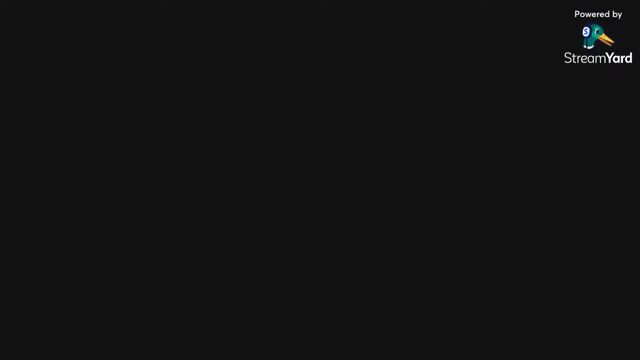 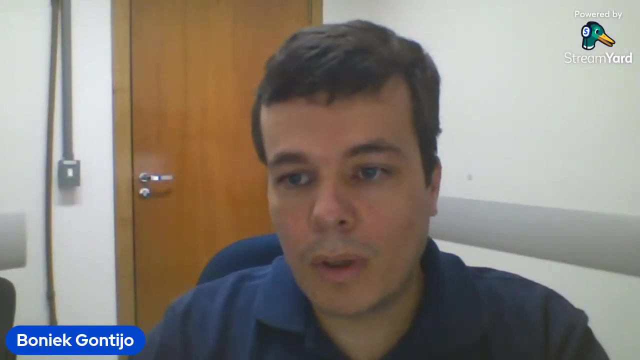 Thank you, Thank you, Thank you. I'm very excited to have you today for one more Alago webinar focused on analytical geochemistry. The Alago webinars are sponsored by Nova Analytica, Thirmo, SANS and FAPERG. 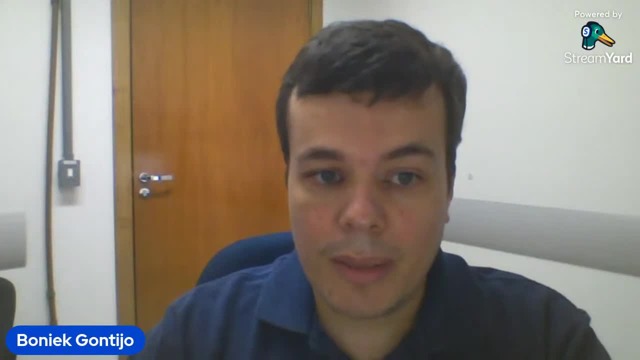 In the name of Alago. we are very grateful to enable this fantastic event. In addition, I want to thank all the organized committee, especially for Vinicio Laércio and Luisa. They are our junior directors that work every webinar on backstage to work hard and provide us this first-rate program. 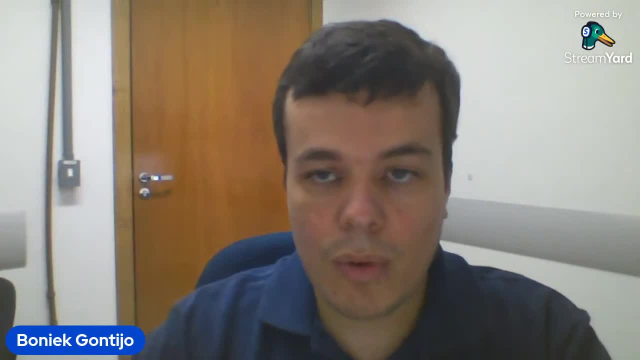 Before moving to our talking, I have a special offer to you. Become a Alago member, Affiliate today, and help this great society become stronger and stronger. Soon we will offer special courses and affiliate members will have special discussions. So hurry up and become an Alago member. 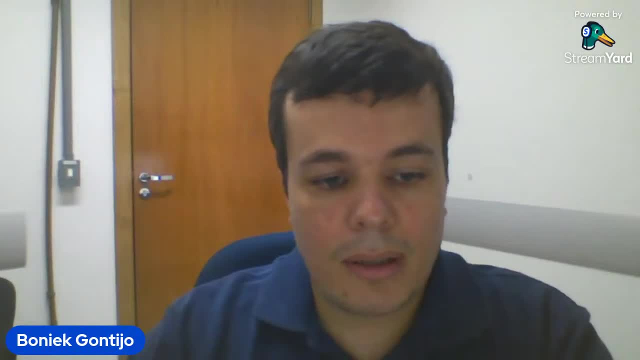 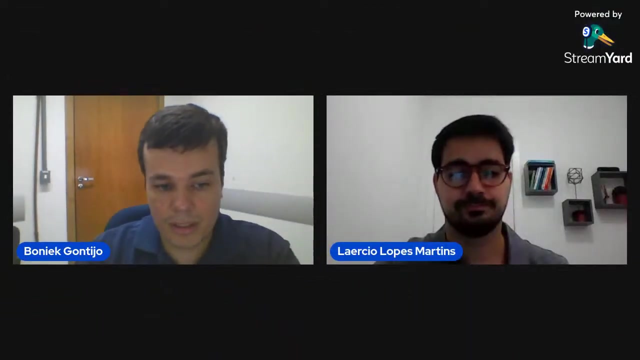 Our talk today is about a new technique, a new methodology to analyze NSO compounds, the FT-ICR-MS, And you'll have a great pleasure to have here today Laércio Machado. Thank you, Boniek. In 2010,, a Master of Science in Petroleum Reservoir and Exploration Engineer. 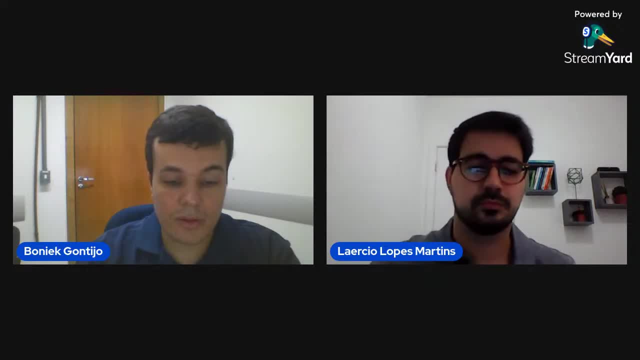 majoring in Petroleum Geochemistry for the North Fluminense State University in 2013, and a PhD in Petroleum Reservoir and Exploration Engineer, majoring in Petroleum Geochemistry, also from UAMPHI in 2016.. He was a professor of the ONG Brazilian Industrial Mobilization Program in 2013 and the Municipal University of Macaé in 2016 until 2017.. 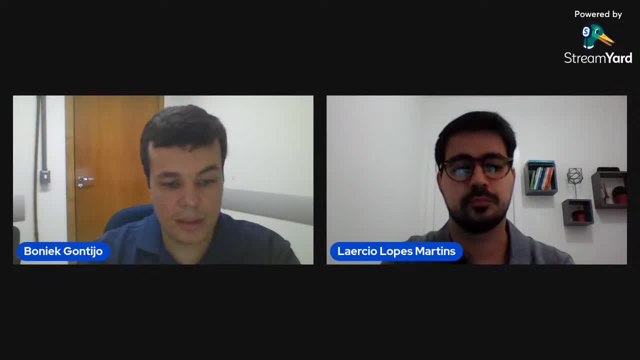 In 2018 and 2019, he spent a year as a post-doctoral researcher in organic geochemistry at GFC, German Research Center of Geoscience Potsdam, Germany. Besides 2013,, he is a geochemist. 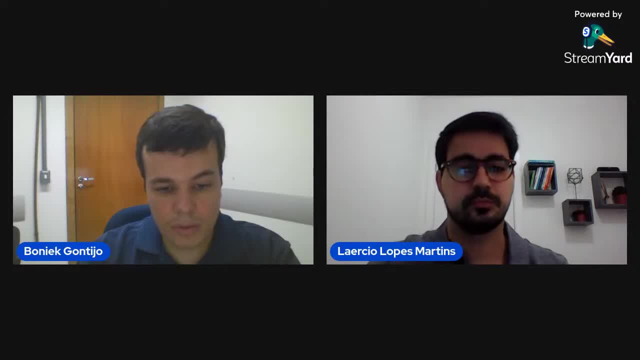 At the Laboratory of Petroleum Geochemistry George Triggs of the LENEP-UAMPH, working as a technical manager, researching projects on organic and petroleum geochemistry and advising undergrads and graduate students. Currently, he is also part of the Board of Junior Directors of the Latin American Association of Organic Geochemistry, ALAGO. 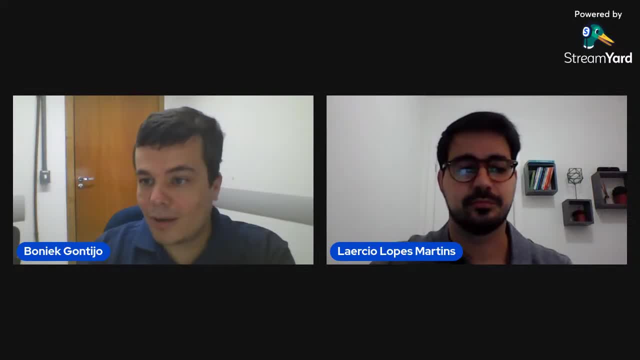 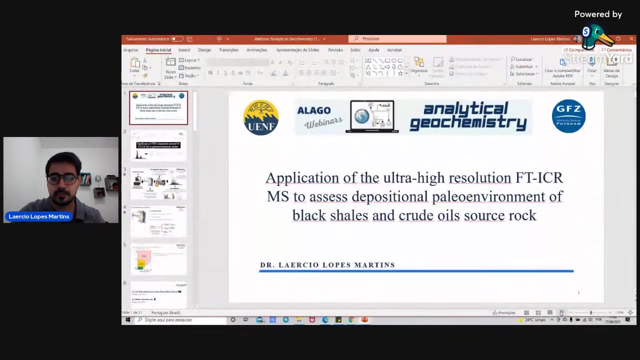 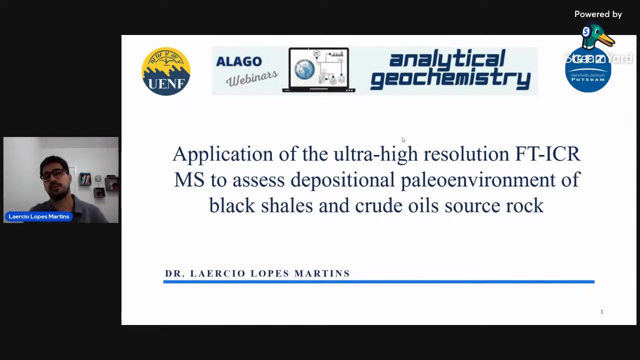 Laércio welcome to ALAGO Webinar. Laércio welcome to ALAGO Webinar. Thank you, Professor Boniek. Thank you to ALAGO for the invitation. So I will open my presentation. So thank you to ALAGO for inviting me. 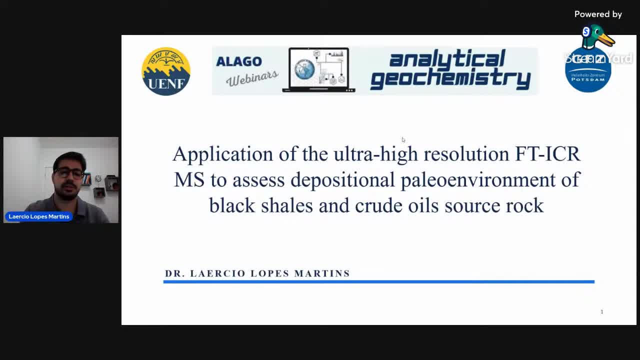 I was honored for that, So it's really good to be here today to share a little bit about this topic that I'm always very, very interested of. That is, the application of the ultra-high resolution FT-SRMS to assess the positional paleoenvironment of black shales and crude oil source rock. 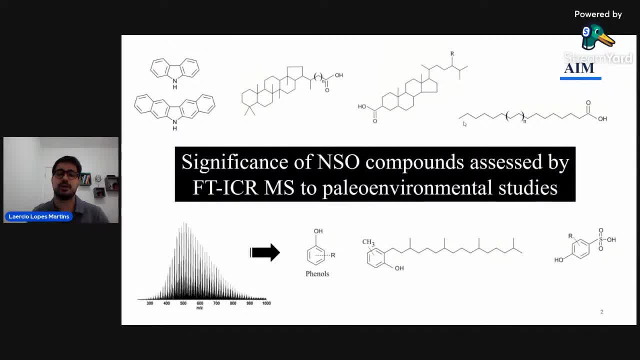 So what is the target of this presentation? So what is the target of this presentation? So what is the target of this presentation? The goal is to show the significance of NSO compounds assessed by FT-SRMS to reconstruct the paleoenvironmentals. 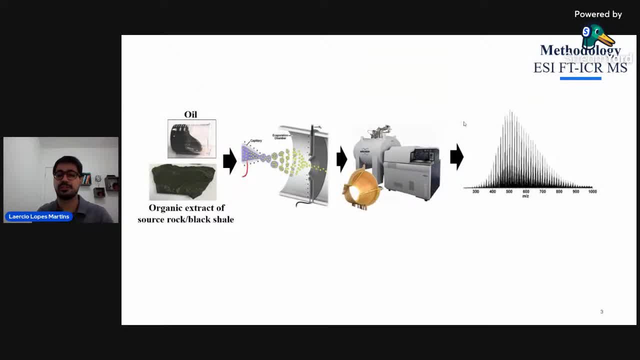 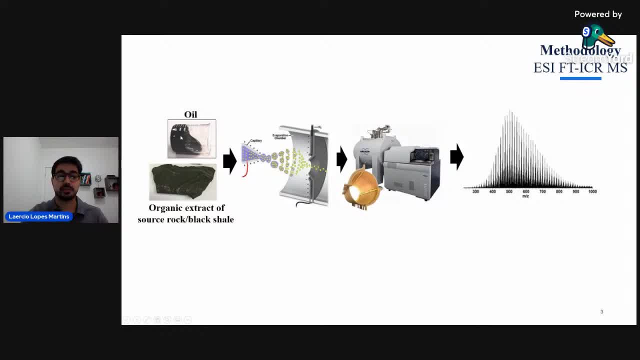 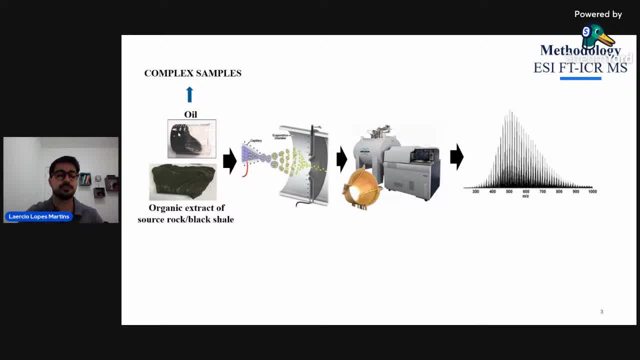 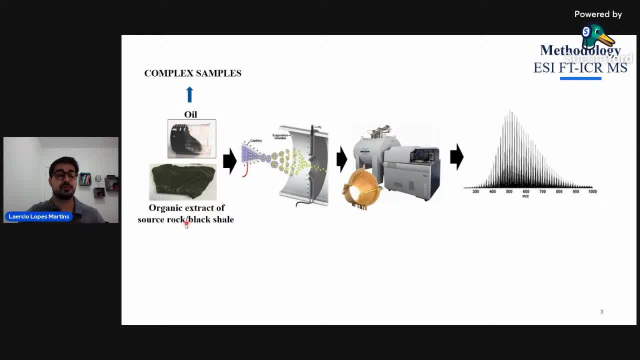 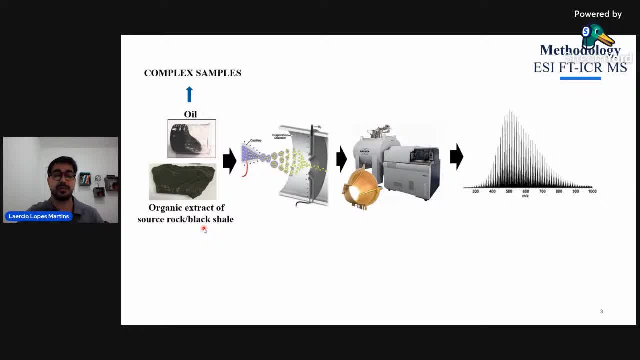 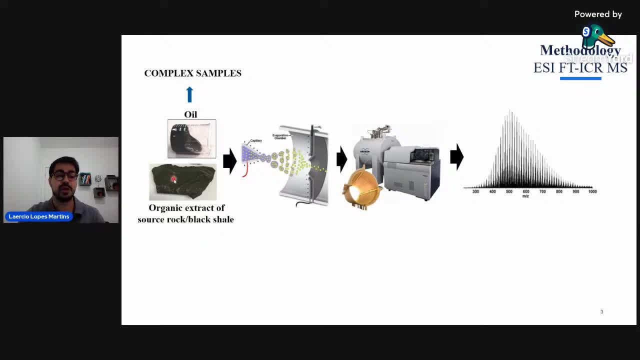 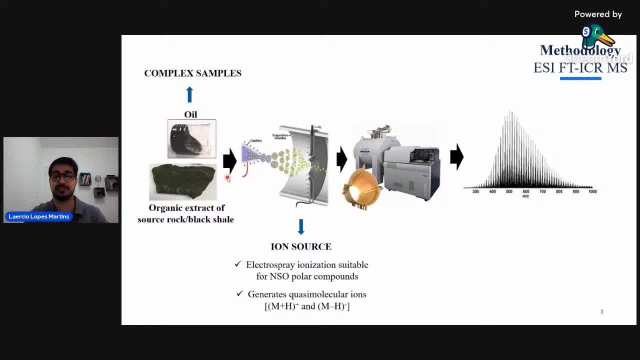 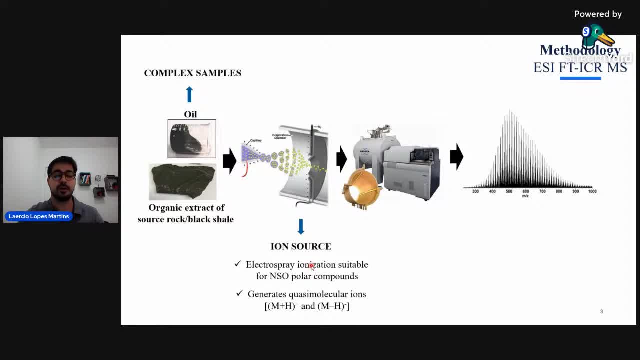 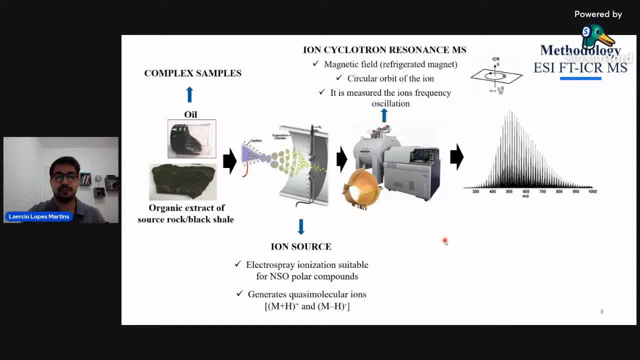 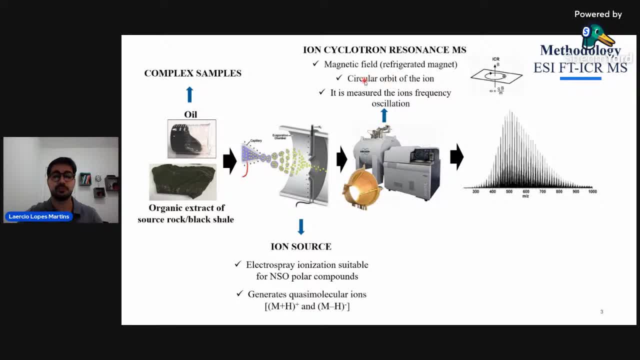 ion is in a circular orbit, So what is measured is the ion's frequency oscillation. that is related to the mass of the ions of the species that we are assessing. So from these masses, in the end we have the mass spectrum, as we can see here. But the thing is we have 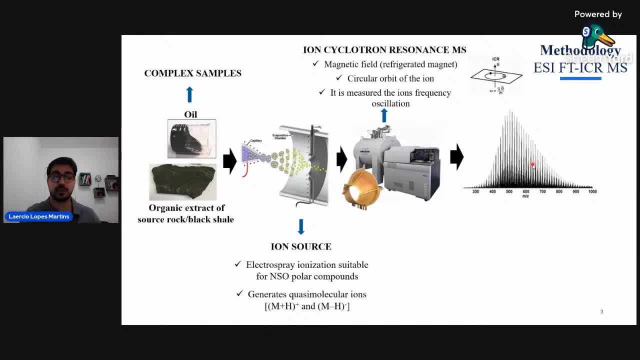 usually a very complex mass spectrum. So what do we do? For example, we have this example from the Smith And a collaborator 2018, that found more than 4,900,000 compounds detected in a half petroleum distillate by 2-1-1 TSLA FTSR-MS. This 2-1-1 TSLA is the equipment with the 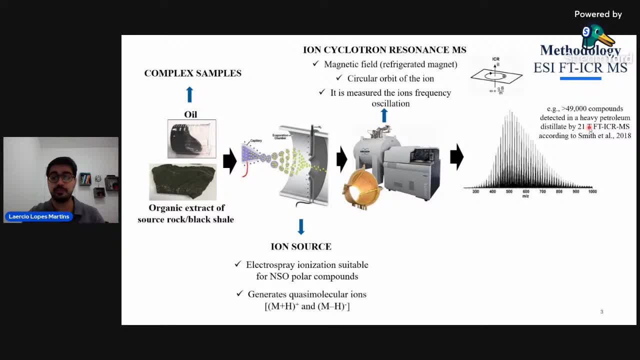 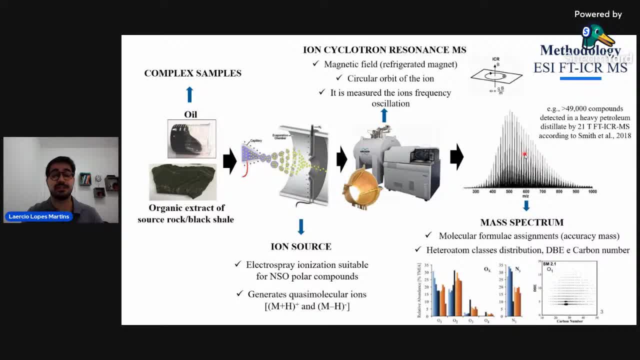 of the molecular formula because we only have the mass. but the mass is very accurate. This Ojfer will do the segment of the ion. This Ojfer will do the segment of the ion. We need to first do the segment of the FTSR–MS. Let's imagine that we have this mass. 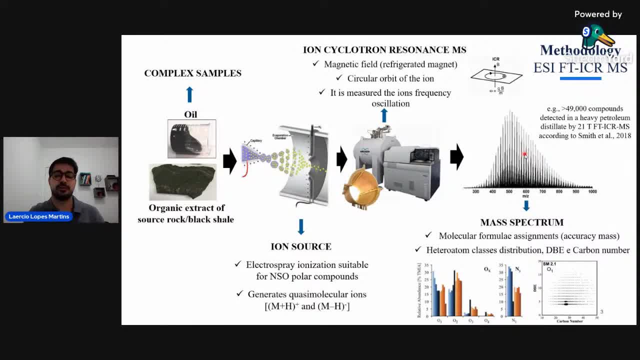 spectrum, 38,000 políticas, and the Hung-Campus system is of a mass with G ει mm. inmates from our team剛 C-HR, a molecular formula 216,129,808, but it is first of a highest form of the mon treasuryt. 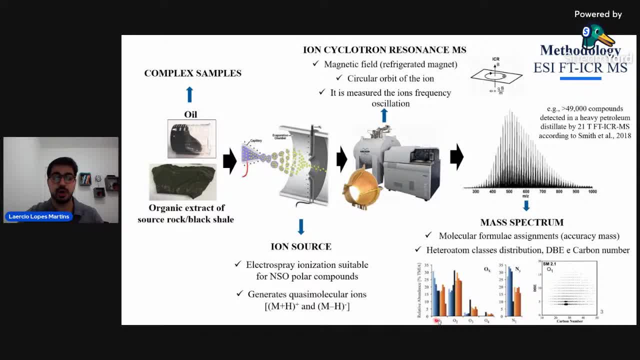 We have the distribution of OX compounds, O1,, O2,, O3, and also the N compounds, And we also have the information about the DBE and the carbon number. The DBE is the double bound equivalent that is linked to the hydrogen deficiency of the compound. 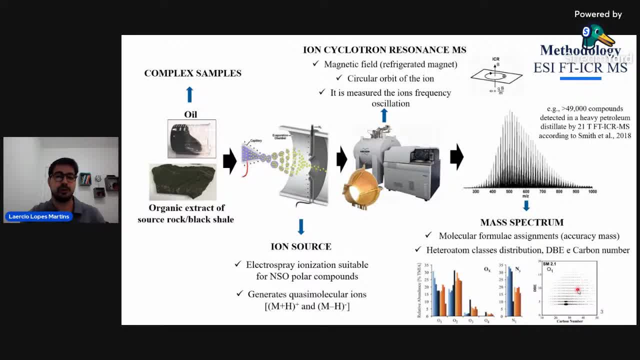 So usually in petroleum omics or in the result reading the data from the FT-ICR-MS, we have this kind of graphics: the carbon number versus DBE. So you can see all the species in this example from the O1 class. 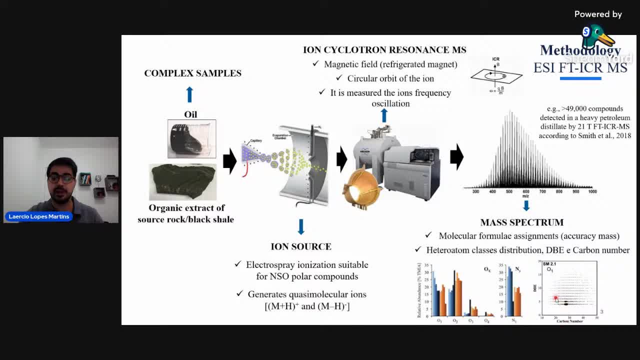 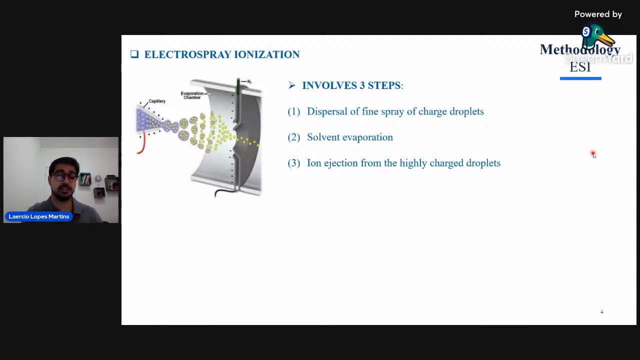 So all the species with the specific carbon number and specific DBE. So this is only analysis And overview, Because what I want in this webinar is to focus on the results from that technique. So another point important that I will only give an overview is about the ionization. 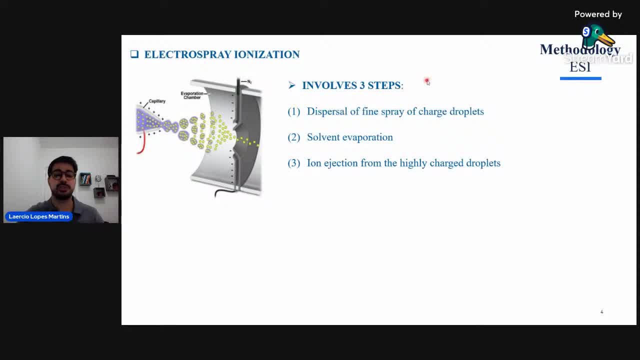 So for the electrospray ionization, it involves three steps. First we have the dispersal of fine spray of charged droplets here, So we have- And then we have the solvent evaporation here And then the ion injection from the highly charged droplets to the mass spectrometer. 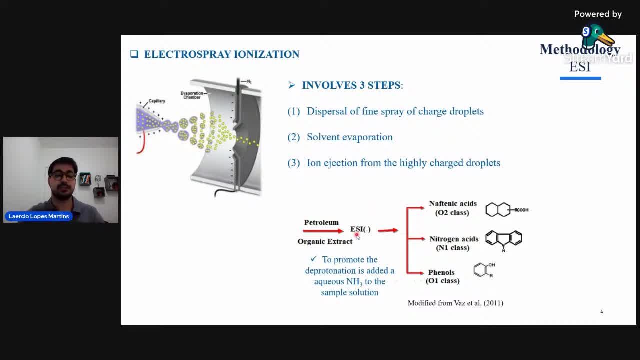 So in the electrospray ionization you can have the positive mode or the negative mode. In the positive mode you usually assess the basic compounds, But in the negative mode you assess The negative compounds. So here is an example which compounds we can assess. 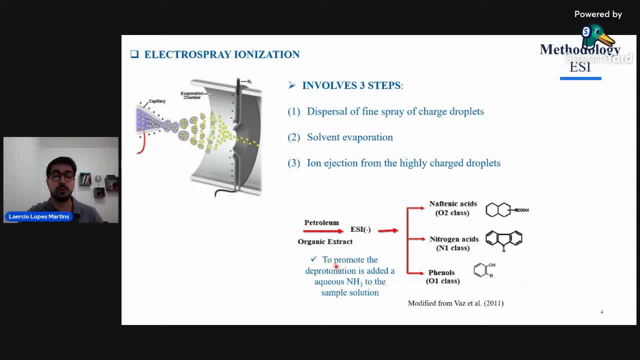 And one important thing is to promote the deprotonation, we need to add NH3 to the sample solution. This is important So you can deprotonate the species. So what we can usually see in this kind Of analysis, using this kind of ionization, is acid compounds such as naphthenic acids from O2 class. 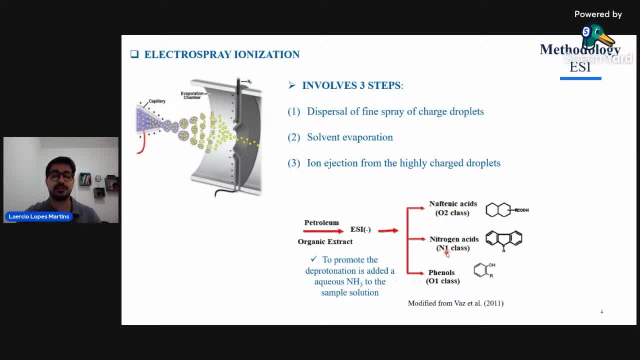 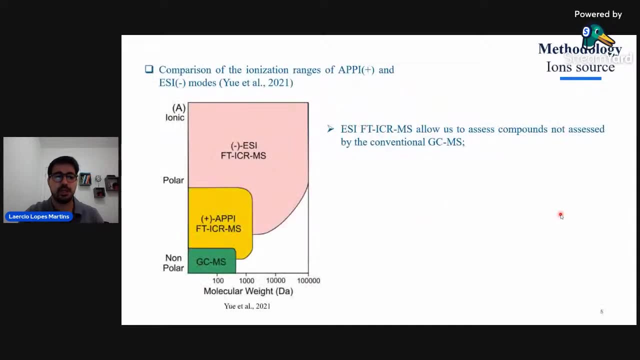 nitrogen acids from N1 class and phenols from O1 class. This is the most that we normally see, but there are others, But this is the most, usually in high abundance. So another important thing- I think it's It's important to show is how great using the EASY FT-ICR-MS is to assess more compounds from petroleum. 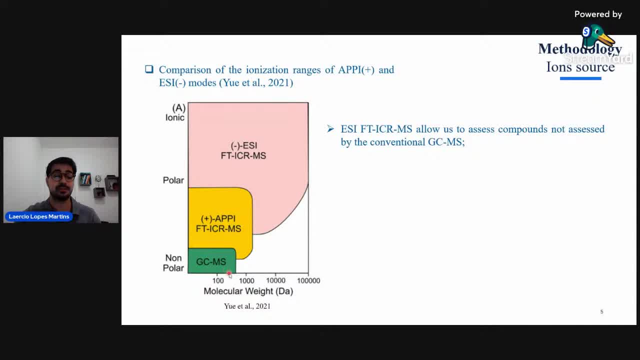 For example, if you have only the GC-MS, it's possible to only assess compounds with low molecular rate and low polarity. But if you have the FT-ICR-MS, for example using the negative mode, electrospray ionization- 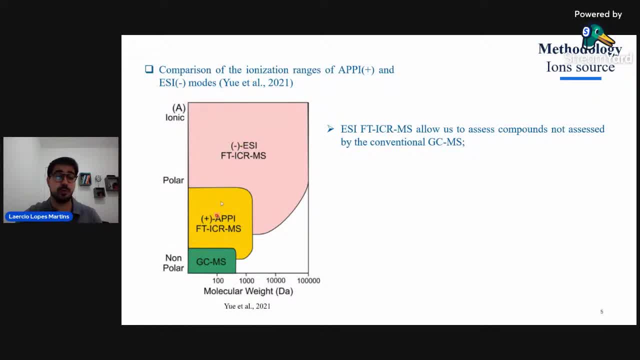 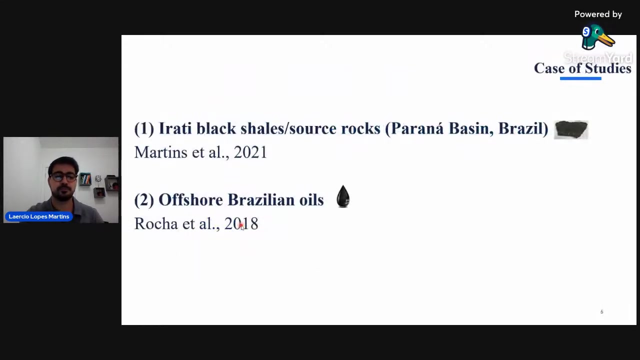 you can assess more polar compounds and with high molecular weight. This is the reason why it's so important and significant this kind of technique, So we can now assess compounds that before you couldn't assess. So in this webinar, I want to show two cases of STERGs. 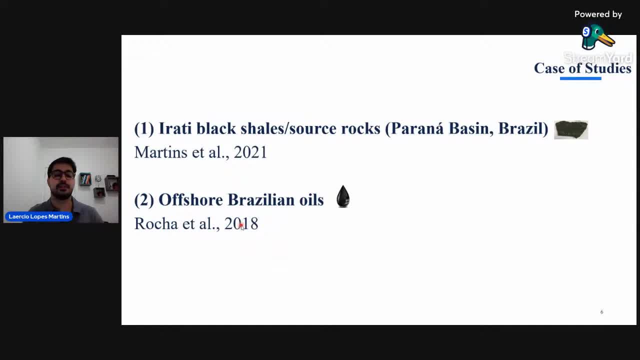 The first of one is the evaluation, the assessment of the paleoenvironment of the Irachi black shales from the Paraná Bays in Brazil. These samples are also source rocks for the petroleum that is in the pyromboid formation, the very half oil that there is there in the tar sands pyromboid formation. 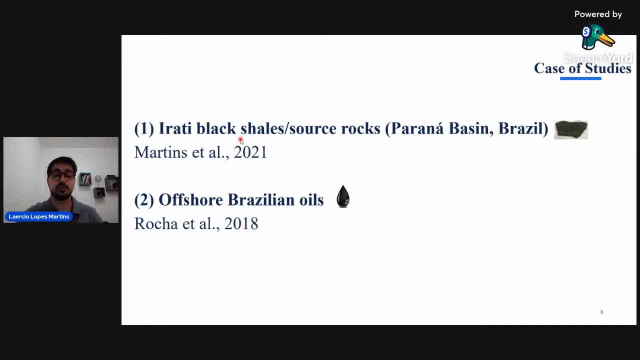 So these results are from my postdoc I will talk about later. And the second case I would like to show you is this publication of Rocha and collaborators- 2018, about offshore Brazilian oils. They do a really, really interesting research investigating the paleoenvironment of the source rocks of these oils. 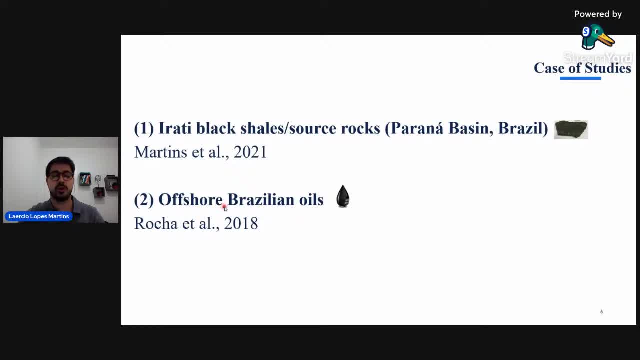 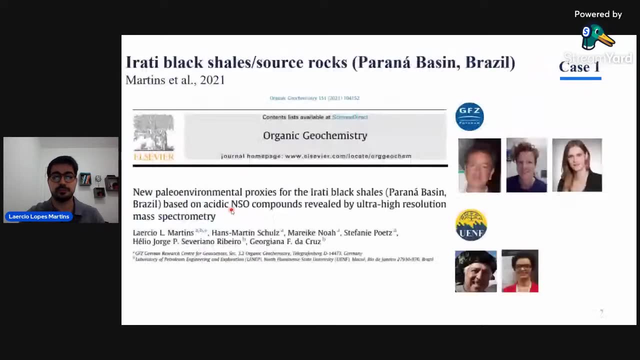 investigating the paleoenvironment of the source rocks of these oils using the FT-ICR-MS. I will present some results from them. So I will show some results from one source rock and another one for the oils. So the first is the Irachi black shales that are also source rocks for the tar sands of the pyromboid formation. 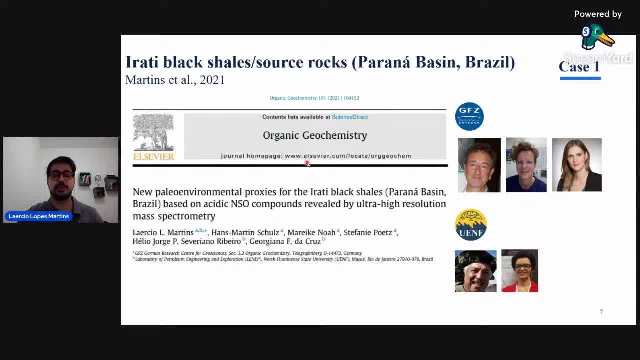 So this work was related to my postdoc at the GFZ. So this work was related to my postdoc at the GFZ. So this work was related to my postdoc at the GFZ In the 3.2 organic geochemical section. 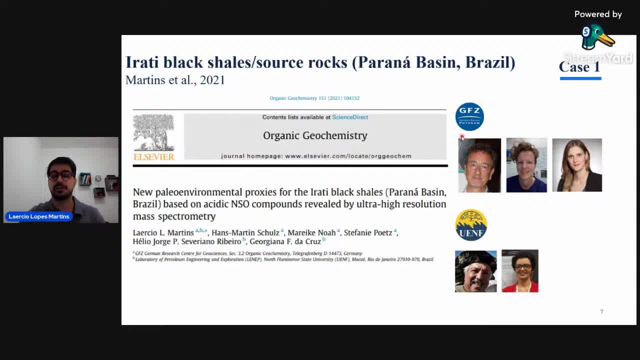 In the 3.2 organic geochemical section. So I was supervised by Hans Martin Schultz. So I was supervised by Hans Martin Schultz, And also I have the collaboration of the chemists there, Staffi Poetz and Maraya Canoa. 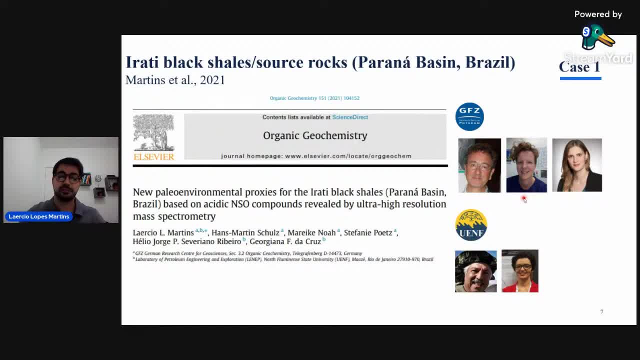 And also collaborators from Brazil And also collaborators from Brazil For this specific publication. we have the geologist Severiano Ribeiro and the chemist Georgiana Feitosa, And also collaborators from Brazil. This paper was about new paleoenvironmental proxies for the irati black shales. 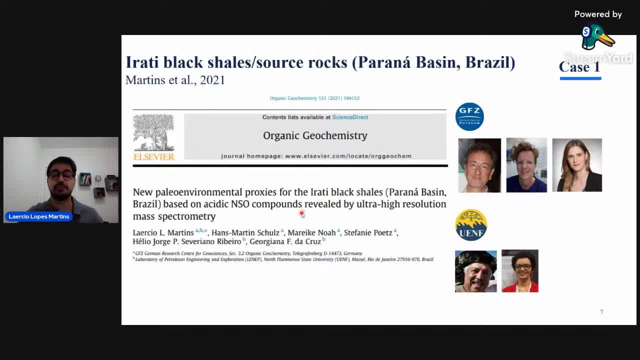 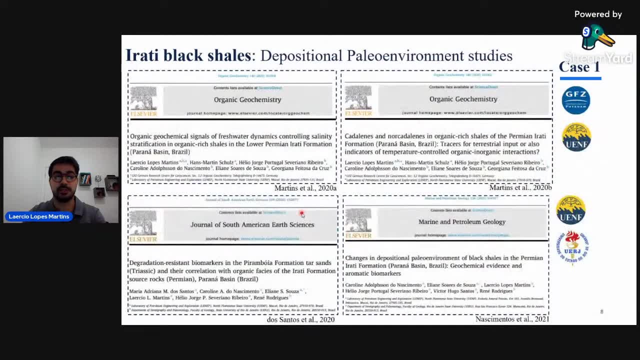 based on acid and estro compounds revealed by the ultra-high resolution mass spectrometry. So I will show you some results from this publication, But first I would like to show you some previous works concerning the irati black shales that give us the base to understand the samples, to understand the paleoenvironmental. 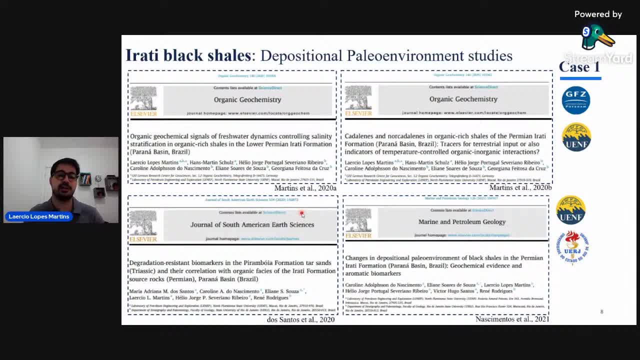 and then we could go deep into FT-ICR-MS results. So here we have four interesting publications about the irati formation, using mostly GC-MS and inorganic techniques. So we have these two first publications on organic geochemistry, about the paleoenvironment of the irati black shales. 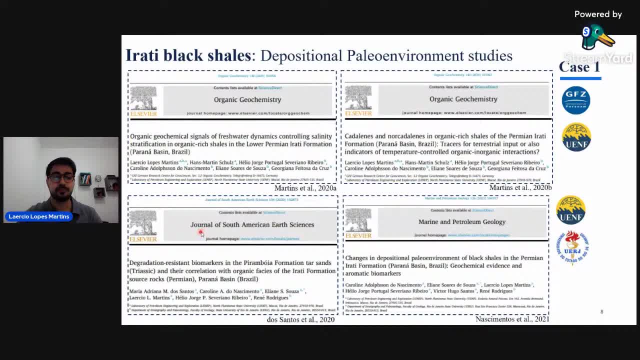 Then we have this publication in the Journal of Sulfur Medical Earth Science. It's related to the master degree of the Maria Adriana, It's about the irati formation and its correlation with the pyromboid formation. And the last one is this one in marine and petroleum geology. 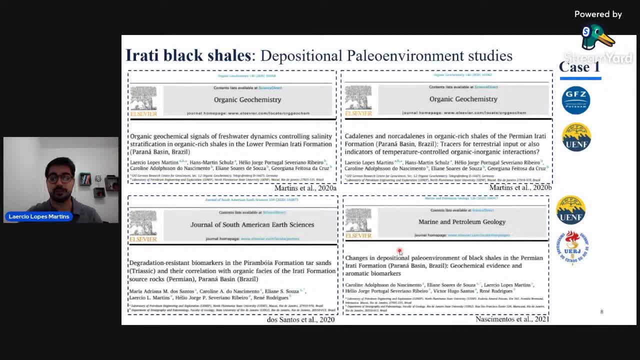 that shows the changes in the positional paleoenvironmental of black shales. It's related to the PAG of the Carolina Dolson in the Nascimento. So it's very interesting and these publications give us the base to go very deep on the petroleum results. 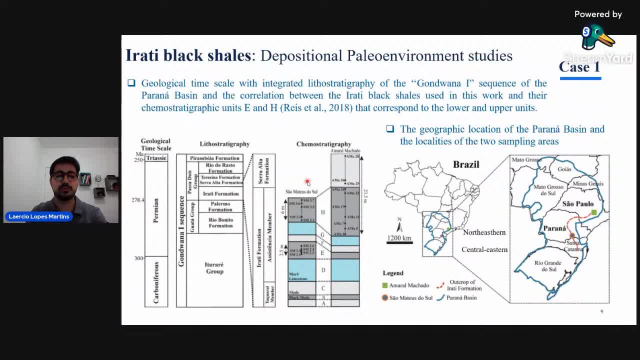 So to talk a little bit about the samples, about the irati formation, So it was deposited in the Permian in 278 million of years ago, as you can see here in this geological timescale and litho-stratigraphy, And here it also shows the chemo-stratigraphy. 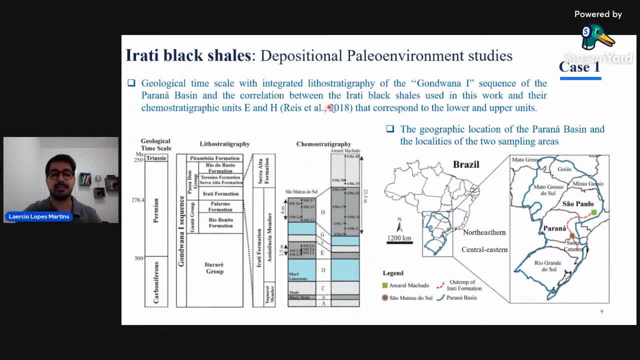 that was made by Reis et al in 2018.. And our samples, our irati black shales, are part of the E and H sections- chemo-stratigraphy sections. So we have in this work- we work with 17 samples. 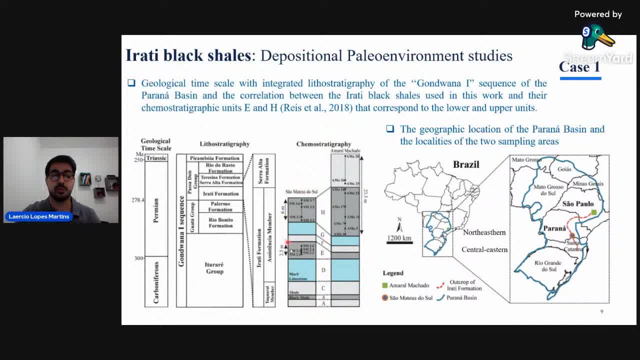 10 from the São Mateus do Sul area here in the central eastern basin, as you can see here, And we have also 10 samples from the Amaral Machado area here in the northeastern basin, as you can see here in the geographical location. 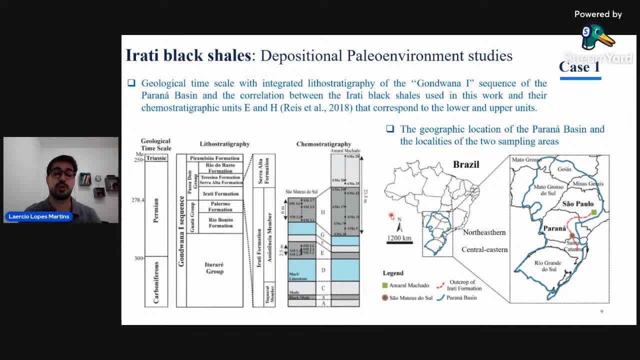 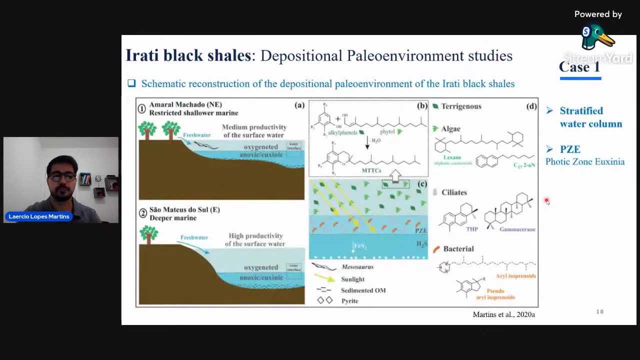 It's also important to say that these samples were collected from the base to the top of outcrops, So it's interesting because we can see how the paleoenvironment conditions change with this. So this is some of very interesting results, I think, from the first publication. 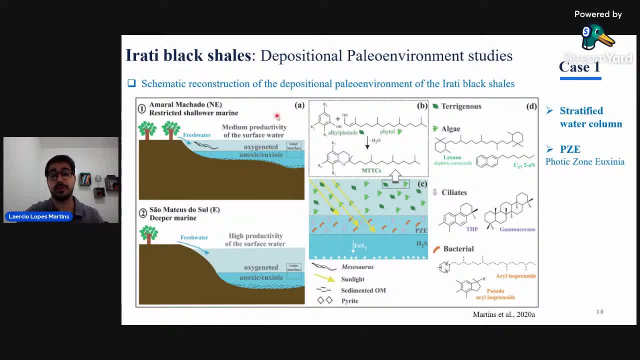 Here we have the idea of the paleoenvironment that we reconstruct. So for the Amaral Machado we have a more restricted shallow marine And for the São Mateus do Sul we have more deeper marine with high productivity of the surface water. 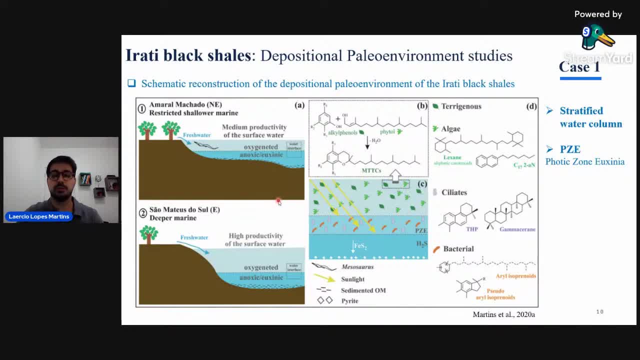 But both of the locations. we could see a stratified water column and also the presence of the photic zone auxinia. We took all this information from mostly biomarkers. If you are interested, you can check more details in the publications, because I don't have time now. 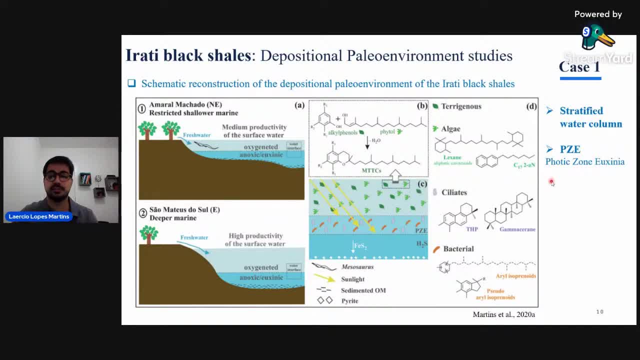 to show to detail this result, but it's pretty interesting So we can see. another interesting thing is there is also some influx of fresh water. We could see that mostly from the Cromans, but also for others biomarkers. So this is how we believe. 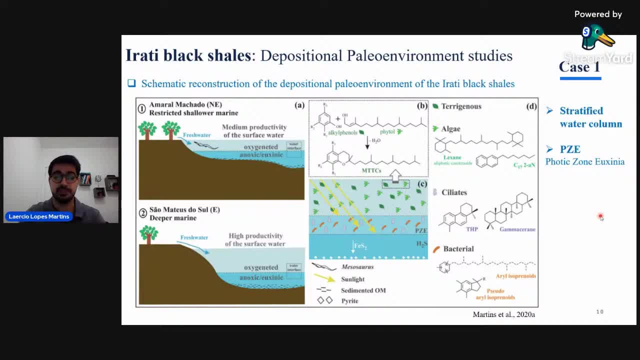 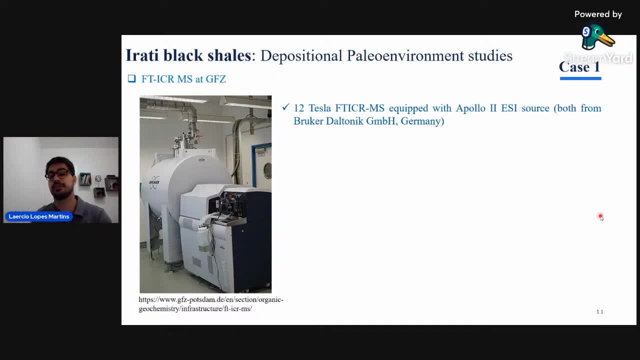 there was the paleoenvironment of the Erich Black Shales, So now I will talk about more the FT-ICR-MS results. I will start with the equipment that was used at the GFC. It was a 12 Tesla FT-ICR-MS. 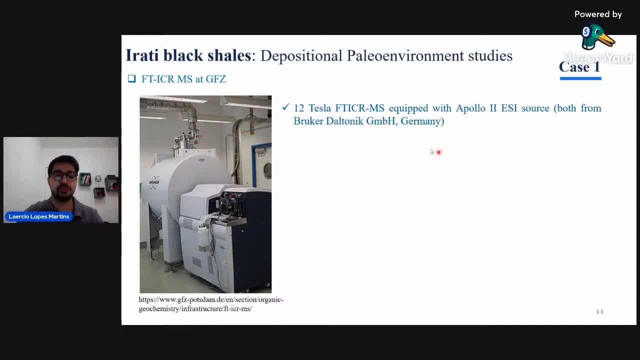 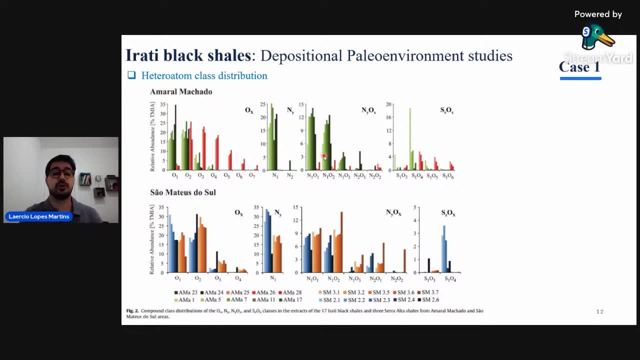 equipped with Apollo 2 ESI, source both from Brugge, Daltonik, Germany. so this is the equipment there. It's a picture from the website of the GFC, And then I will start with the ethereatome class distribution. 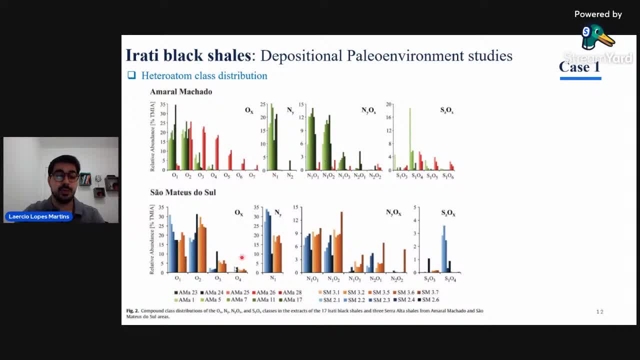 as you can see here. So we have here the distribution for the samples from the Amarão Machado area and here the distribution of the samples from the São Mateus do Sul area. So here we have 10 Erich samples and for Amarão Machado we have 7 Erich samples. 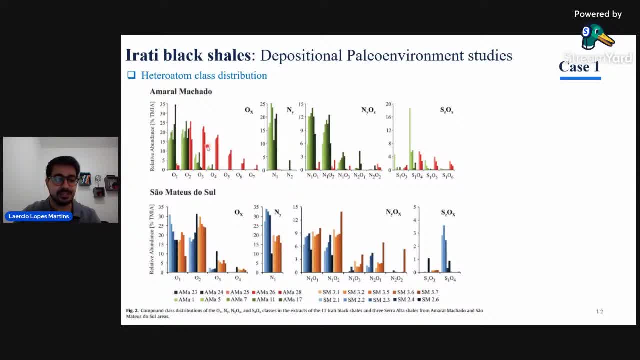 In addition, we have 3 samples- that is here in red- that are from the Serra Alta Formation. It's an overlaying formation of the Erich. I will explain a little bit about why we included this formation, these results, in this work later. 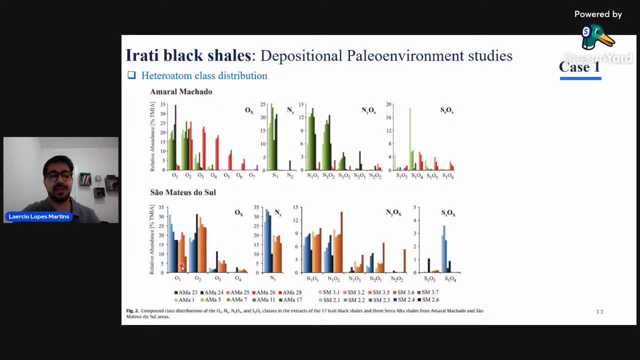 So what we can see here- and it's very interesting- is that there is some difference between the composition of the samples. As you can see here, for example, the O1 class diminish with the direction of the top of the outcrops. 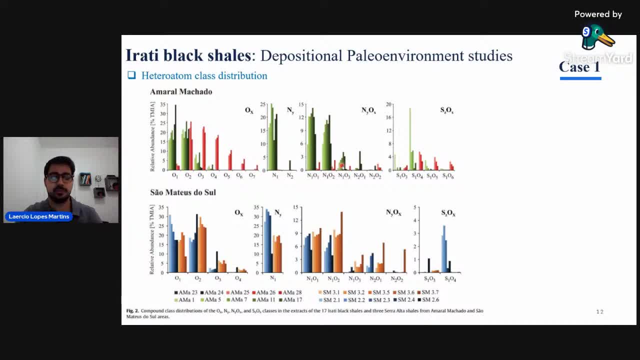 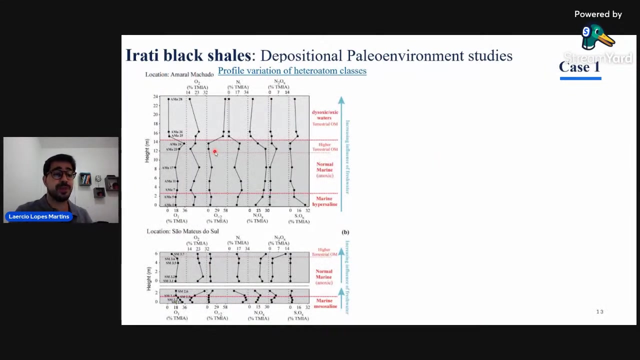 and a lot of really interesting information here, But one that I want to highlight is the high amount of the O2 compounds here in the Serra Alta Shales. I will explain why this later. So from another perspective, I would like to show the eteratome classes. 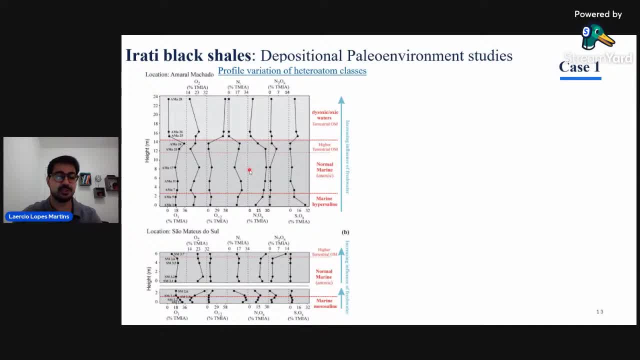 the variation in this profile, because here we can see better how the eteratome classes change with the height of the outcrops. So what we can hear in the right side it's the reconstructed paleoenvironment for the previously. 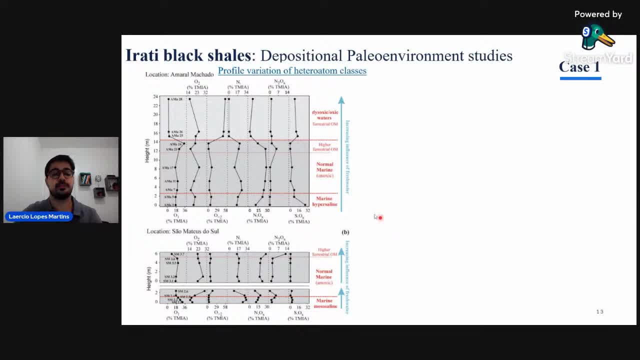 previous publications. So, for example, here in Amaral Machado, at the base we have more marine hyperselene and with the increasing flux of freshwater it's in the top. we have more normal marine with high terrestrial organic matter and the Serra Alta Shales. here 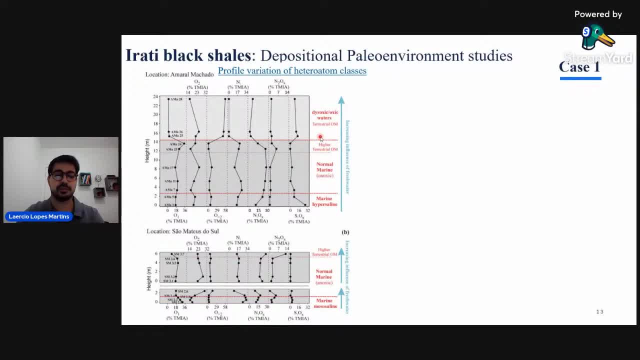 has a deoxy-oxy water and a lot of great terrestrial input of organic matter, And it's kind of similar for the São Mateus do Sul. So from the eteratome classes variations, what it's interesting to show here is the high abundance of NU1 compounds. 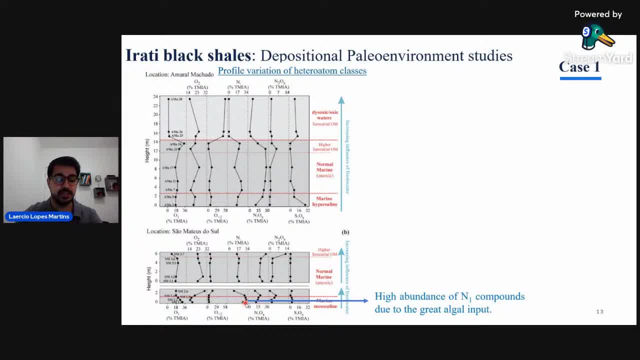 due to the great algae input here to the base of the São Mateus do Sul. This is pretty interesting, this high abundance, because these first samples from the base we could see from the biomarkers that it was a blue algal in this. 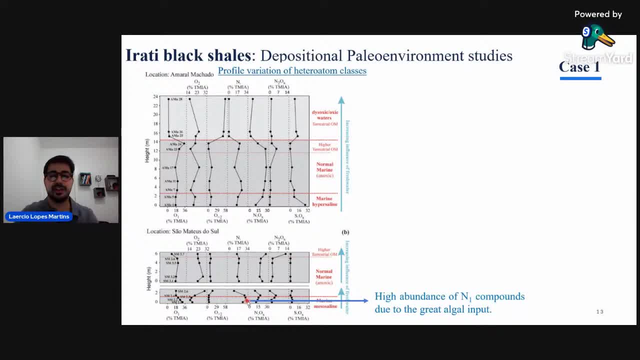 a high amount of pristane and phytane, really really high. So it's interesting that they also have high abundance of NU1 compounds And also interesting it's here, from the base of the Amaral Machado, we have high abundance of SO compounds. 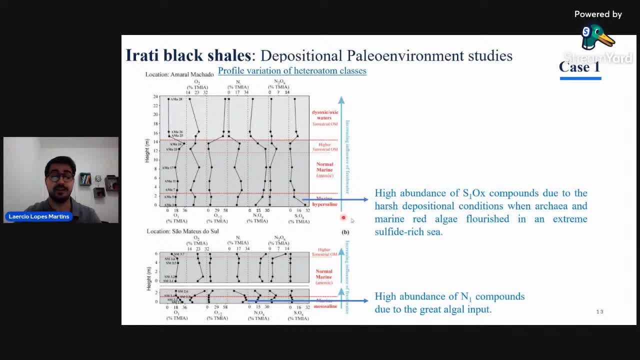 due to the harsh depositional conditions when archaea and marine red algae flourish in extreme sulfate rich area. So here, as you can see, we have a high amount of SO compounds. These results come from the first publications, And here from the Serra Alta. 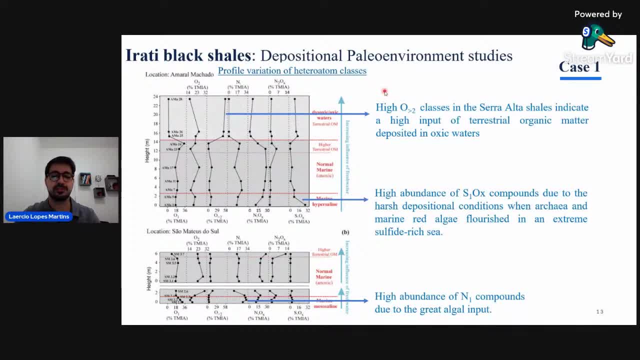 we have high amount of O compounds that indicate a high input of terrestrial organic matter deposited in oxki waters. So from these results we could think that this variation could not be related only to the paleoenvironment conditions, but also, for example, 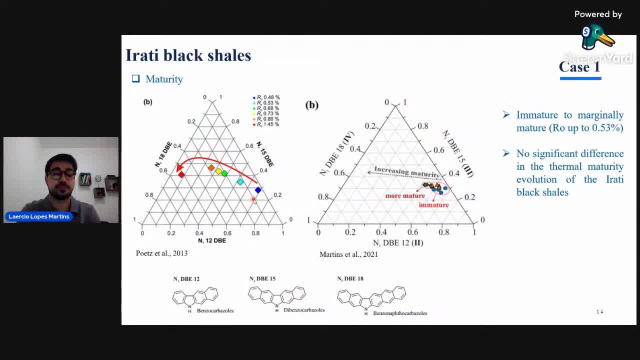 from the maturity. So that's the reason I want to show these results also, that it's from the maturity of the Irachi Black Shales. Here in the left, in the right, in the left, we have the results from the. 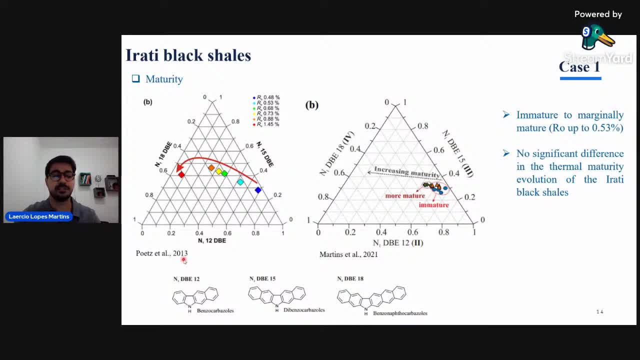 Boets and Collaborators 2013, that they suggest this type of diagram using carbazoles, using benzocarbazoles, d-benzocarbazoles and benzonaftanocarbazoles to assess the maturity of rocks. 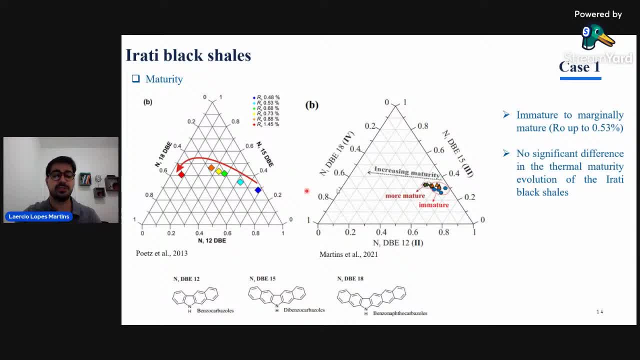 of source rocks. So what we see when we check our samples, our Irachi Black Shales, is that they are in the very immature area, as you can see here. If we compare these two graphics, we can see that our samples is in the area of. 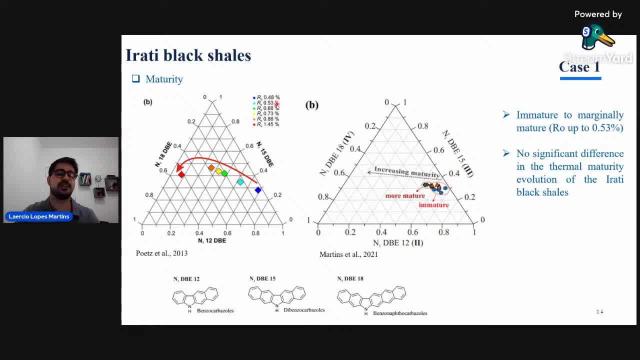 0.48 to 0.53 reflectance of Victorinite reflectance. So this is a very low maturity. So we can see here that our samples, the Irachi Black Shales, don't have some difference in the thermal maturity. 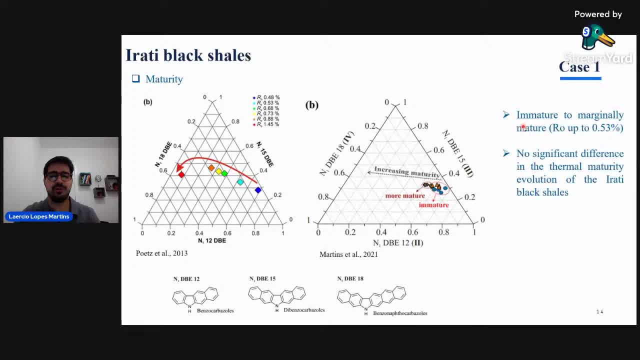 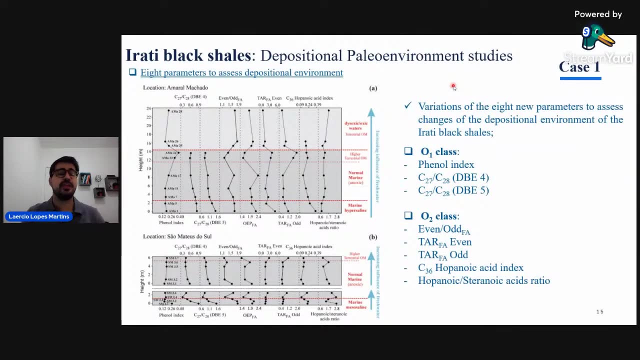 and also are very immature to only marginally mature, And this is in agreement with our other studies from the biomarkers and for the rock eval analysis. So I think the most interesting result for this publication is the eight parameters that we suggest, as you can see in this figure. 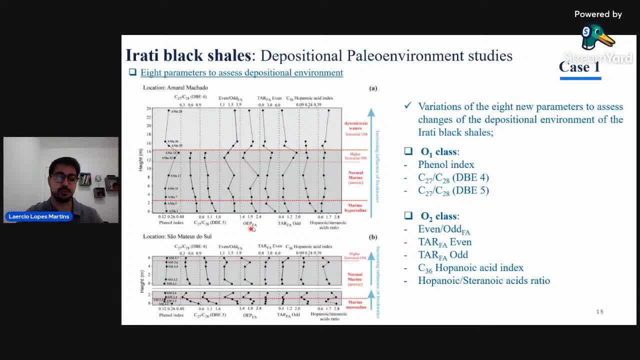 Here we have nine, because it also shows one parameter from another publication. So we have all these parameters, for example, and they are basically based on the O1 class and O2 class. So from the O1 class we have the phenyl index. 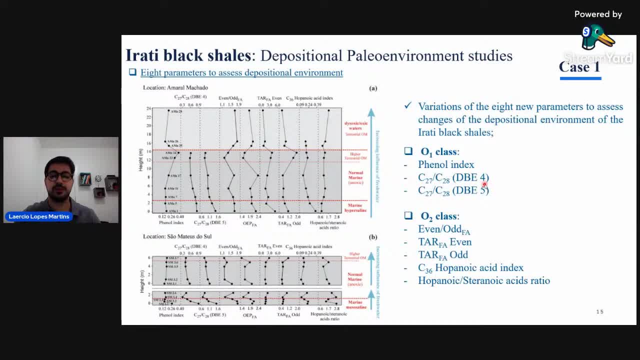 and two parameters based on the isoprenylglyphenols. And for the O2 class, we have three parameters based on the fatty acids, the acyclic acids and other two parameters based on the hopanoic and stearanoic acids. 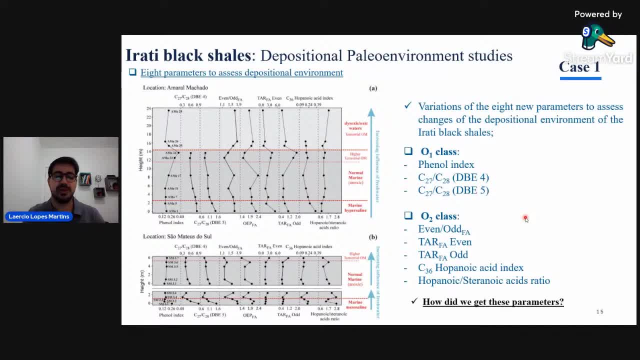 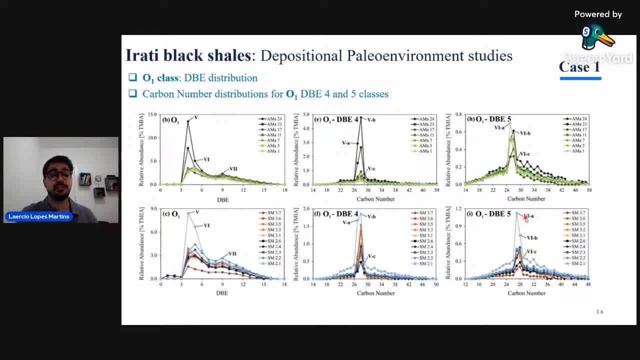 But how did we get these parameters, Where they came from? I will show you how we achieved that. So I will start with the O1 class. So here we can see the distribution, the DBA distribution, of this class for the Amarão Machado area. 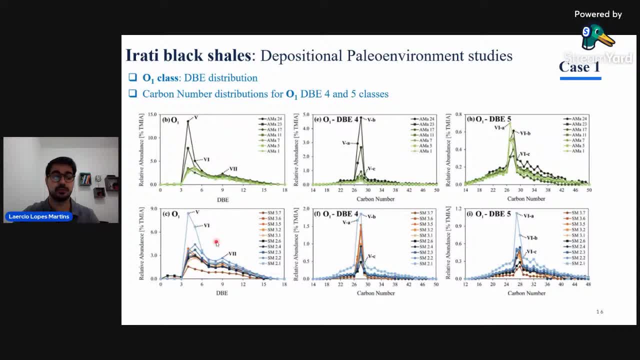 and for the São Mateus do Sul area. So it's interesting to see the high abundance of compounds with the BF4 here and also the BF5 here, mostly for the samples 23 and 24 at the top, at the top of these outcrops. 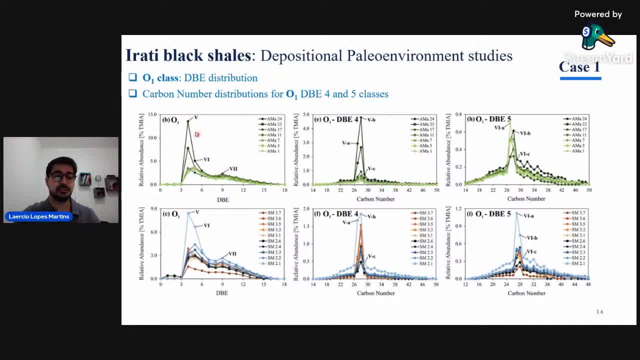 So what we did is take this DBA and did and obtained the carbon number distribution. So here we can see the carbon number distribution of O1 compounds with DBA4. And in the right we can see the DBA, the O1,. 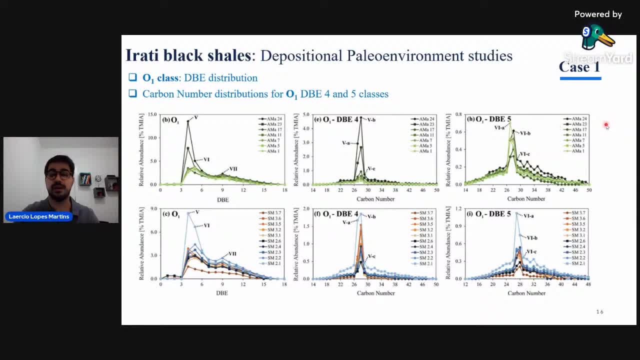 the carbon number. distribution of O1 compounds with DBA5.. What was really interesting is the high abundance of compounds with 27 and 28 carbons. This was really interesting for us. This could be the isoprenylglyphenols or some esterols. 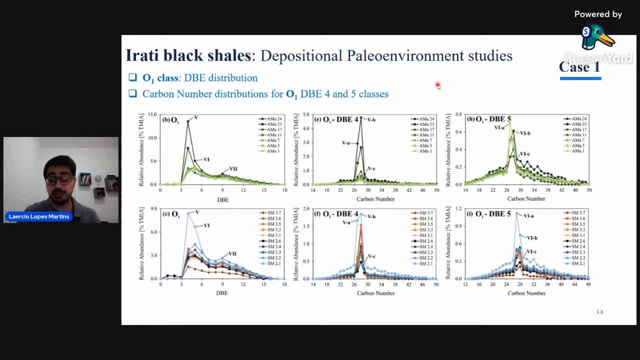 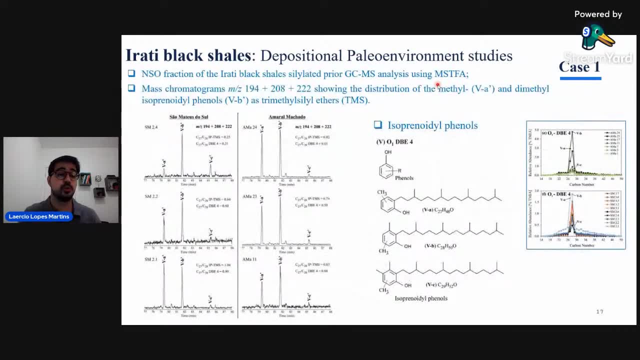 There are these two possibilities from the literature, So we want to be sure what kind of compounds were. So what we did was we take the NaSO fraction of the iridoblack shells and solute it using the MSTFA. prior GC-MS analysis. 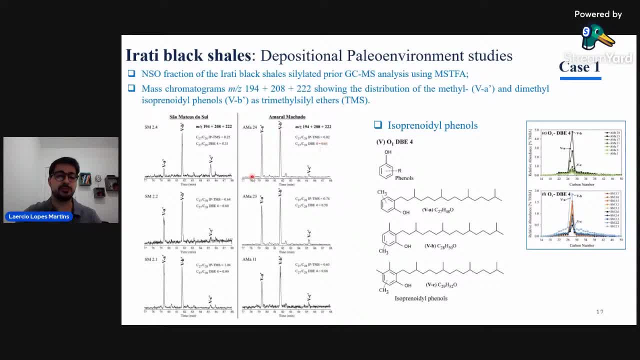 And then we look for for the isoprenylglyphenols soluted and we find it. So what we can see here is the mass chromatogram MZ149, MZ194, MZ208 and MZ222 in the distribution of the methyl. 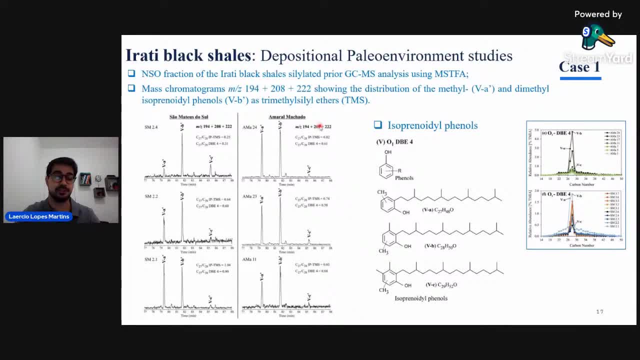 and dimethyl isoprenylglyphenols as trimethylsilyl ethers. So it was really interesting for us that we could be sure now that the isoprenylglyphenols are in the samples. They were detected in the samples. 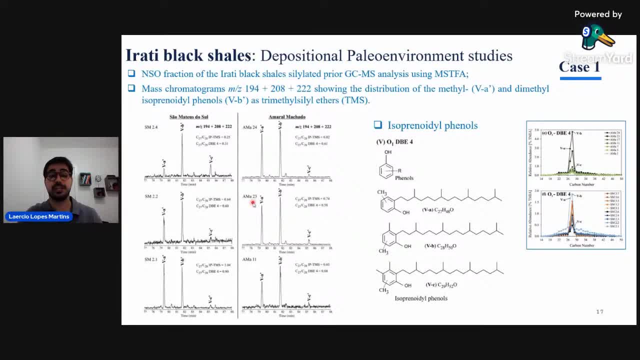 And another interesting thing was we did some correlation with the ratio between the 27 carbon over the 28 from the GC-MS results with the results from the FT-ICR-MS and they correlated very well. For example, here for this sample. 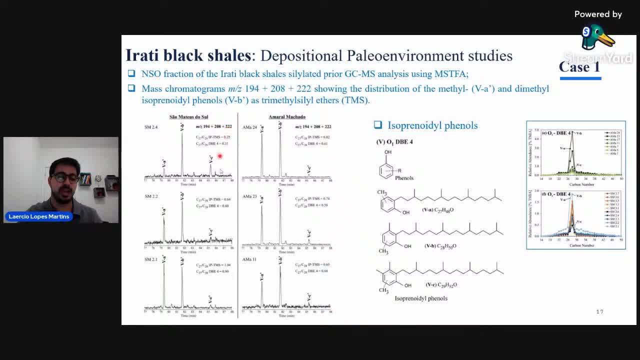 we have low ratios and for the base sample we have very high samples, like one And the same for the Amaral-Machado. we have here high values and in the base the low values. So they correlated very, very well. So now we are more sure. 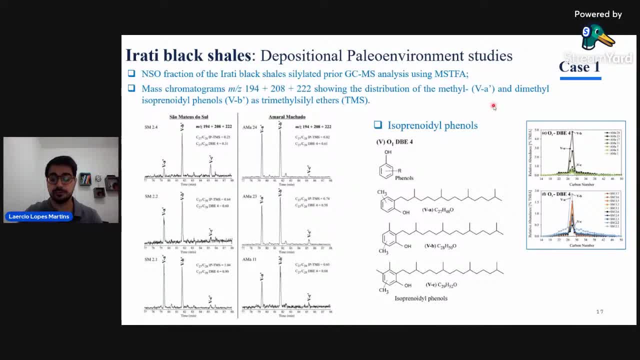 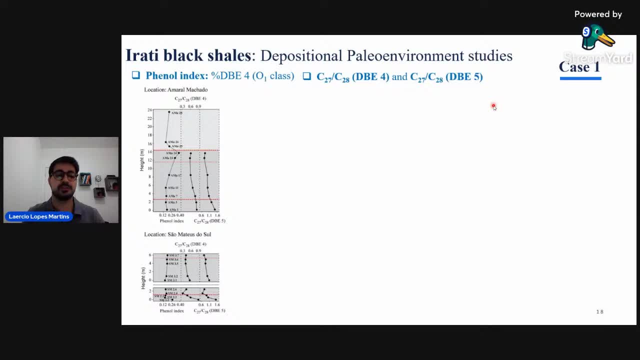 that these compounds are the isoprenylglyphenols, So from the O1 class we suggested three parameters: The phenol index that is based on the percentage of DBF4 class DBF4 compounds, and also two parameters based on the isoprenylglyphenols. 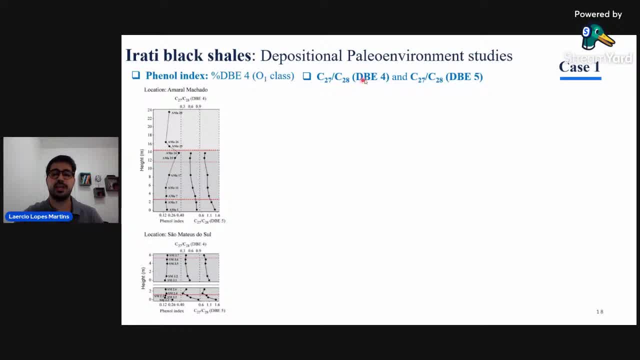 So the C27 over the C28 for DBF4 and for the DBF5.. So here is the profile for these parameters over the height of the outcrop. So what is interesting to show here is for the phenol index we can see high values. 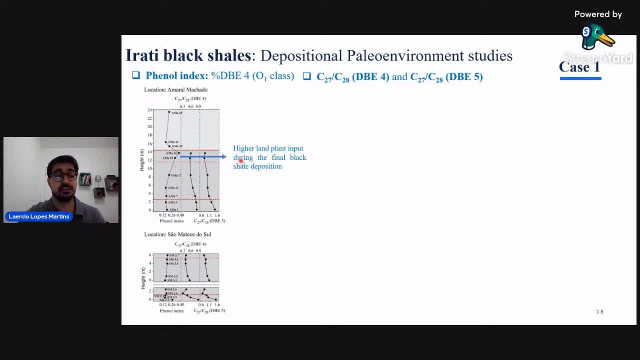 for the top samples here. that showing that is related to the high land plant input and also pretty interesting, it's the high abundance here in the base of the São Mateus do Sul that we already saw in the other publication: a high influx of fresh water here. 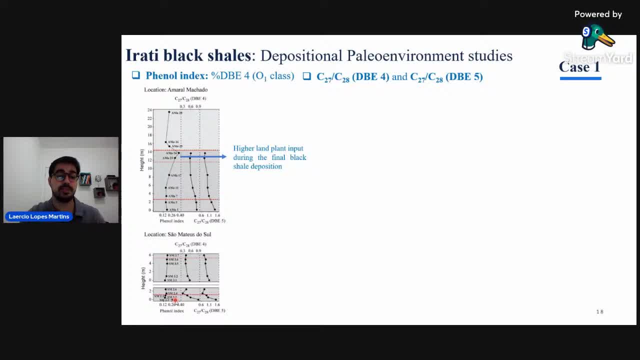 with the algal albun and probably a high land plant input. So from the from the ratios based on the isoprenylglyphenols. it's really interesting here in the base that we can see here in the base of the Amaral Machado. 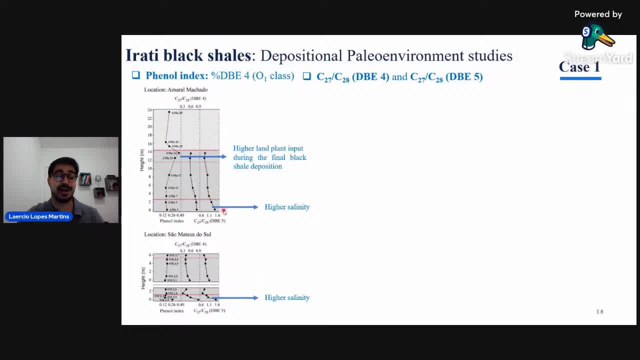 and São Mateus do Sul that they have high values. that is related to the highest salinity. So with the increasing of the salinity we also can see the increasing of these ratios. So they can be used to paleo to assess paleo salinity. 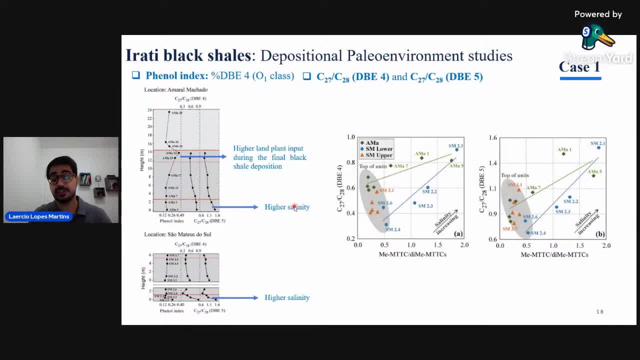 It's pretty interesting. And other interesting result was the correlation between these two new parameters with the parameters using the methylchromase from the GCMS. So here we have the methylchromase over the G-methylchromase. So what we can see. 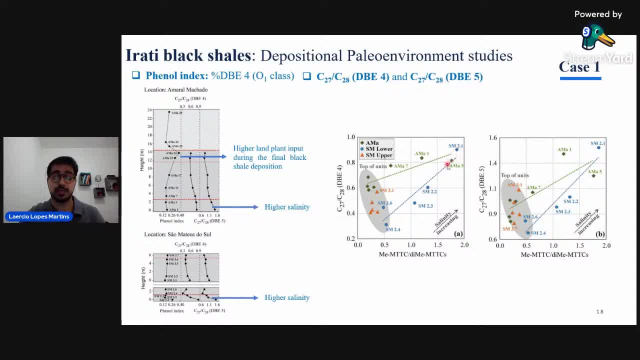 it's a very good correlation- not very good, but a good correlation between them. and here the methylchromase are usually high in more in samples normally deposited in high salinity environments. So with the increasing of this, of this ratio, we have the increasing the salinity. 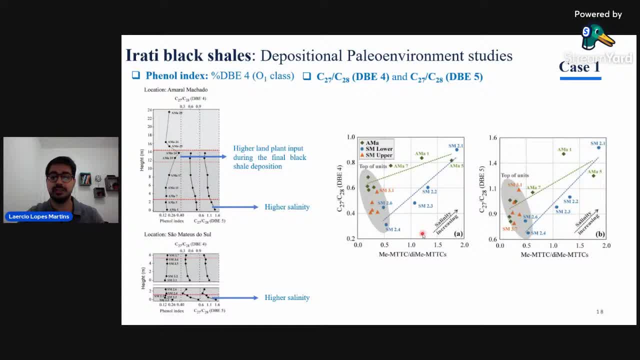 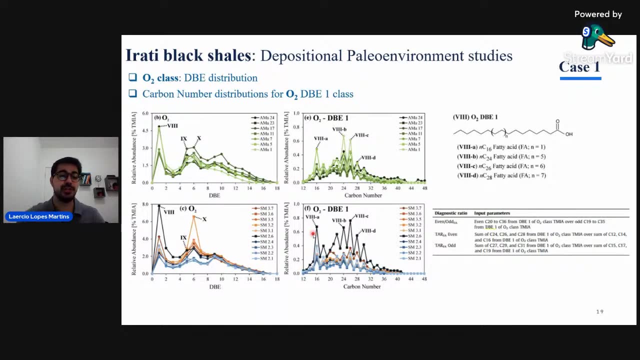 as for the suggested parameters. So we can see here a good correlation between them and that these parameters could be useful to assess paleo salinity. Now I will talk a little bit about the O2 class. So here what we have in the left: 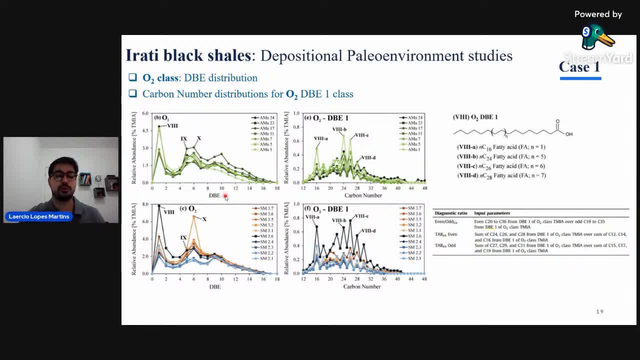 is the DBA distribution of O2 compounds. So what we can see here is the high abundance of compounds with DBA1- here that are the fatty acids, as you can see here in the right. So- and also high abundance of compounds with DBA5. 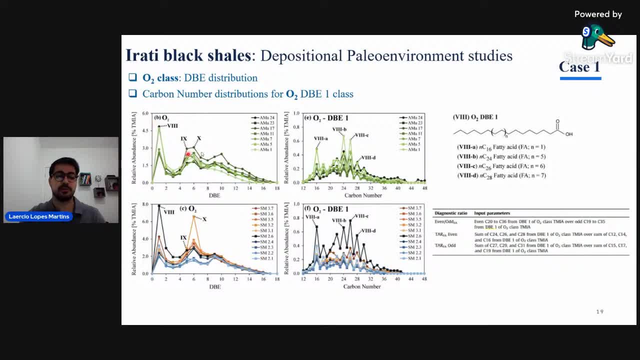 and 6.. So this was some compounds of that take our attention. So at first I will show the carbon number distribution of the DBA1 compounds, the fatty acids here, But we can see at first. it's very interesting the profile with some odd. 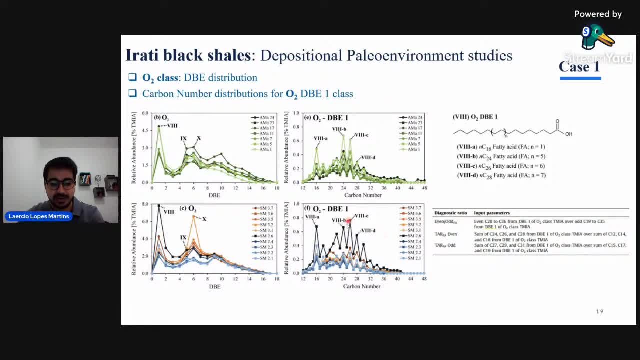 over. so it's very interesting. and we can see also some high abundance of specific compounds, like here 24,, 26, 28.. So, based on this distribution, we suggest three new parameters and also take in account the some parameters from the biomarkers. 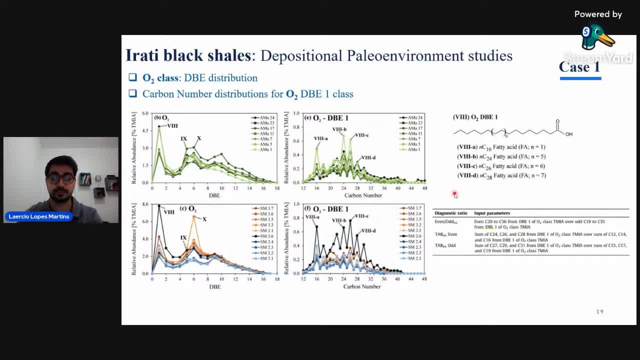 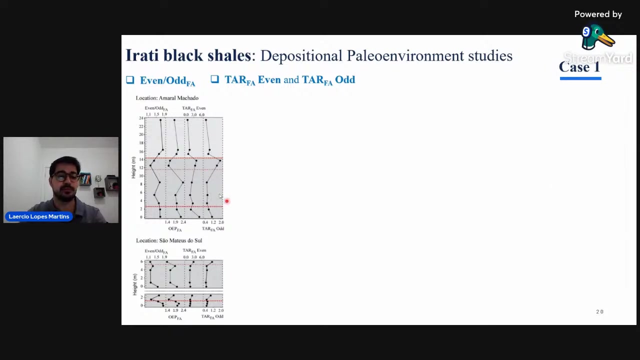 And also that the original echoes Rachel for the fatty acids using the even and the odd acids, as you can see here. If you want to see more detail, you can see in the publication how they are calculated in detail. So it's interesting to see. for the 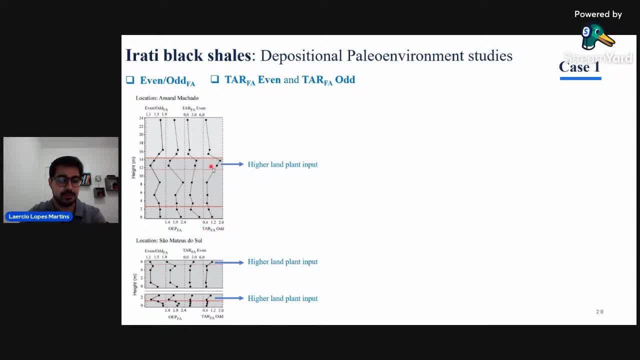 original echoes Rachel for the fatty acids, the high abundance, the high values for the samples at the top of the locations of the outcrops. This is probably due to from the GCMS that the original echoes Rachel, from the hydrocarbons We can see. 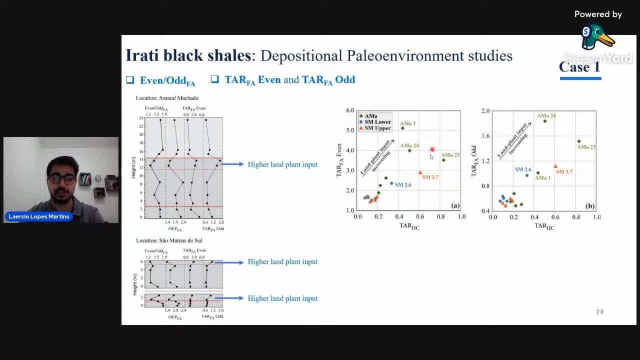 some kind of correlation. This was also really interesting for us. So for example, that samples for the top of the outcrops like 23, 25 or SM 3.7. we can also see high values for AMA1.. AMA1 is in. 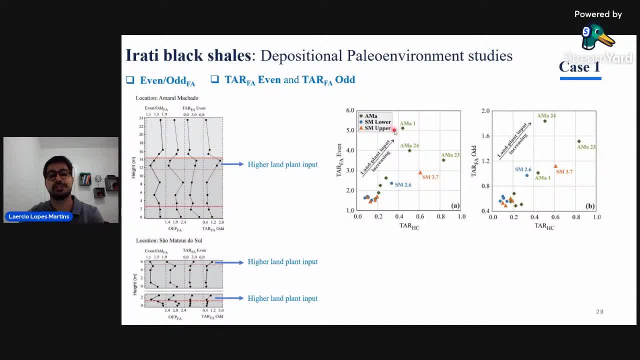 the base is here in the base of Amaro Machado. This is probably because this sample was deposited in a very proximal environment with more influx of carbon, So we can see that this is a very high value of carbon. So we can see. 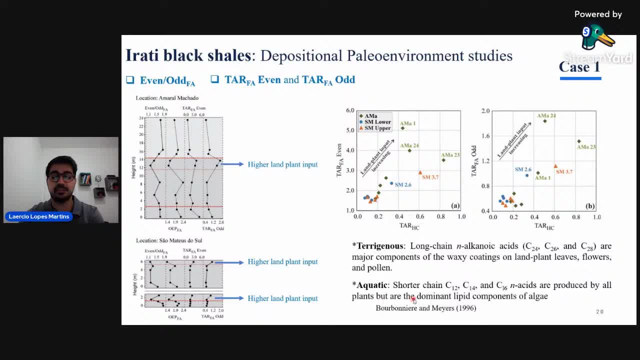 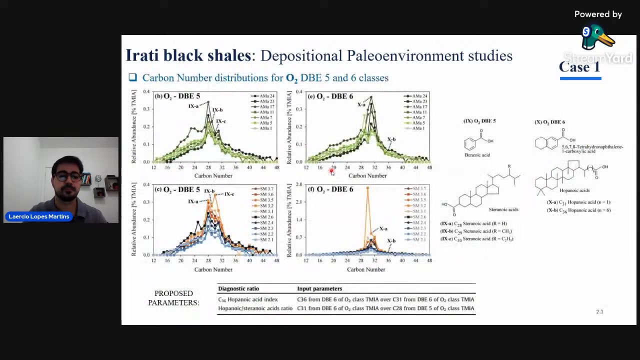 that this is a very high value of carbon. So we can see that this is a very high value of carbon. So this is a very high value of carbon. So we can see that this is a very high value of carbon. So we can. 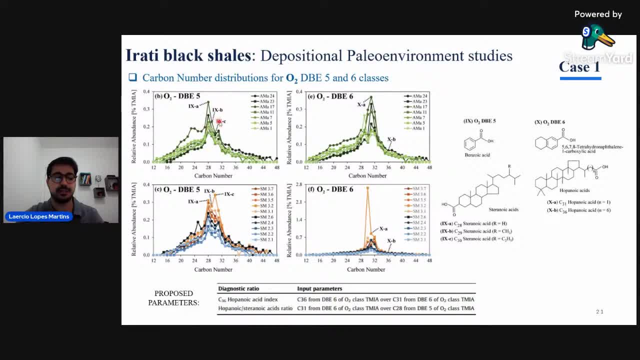 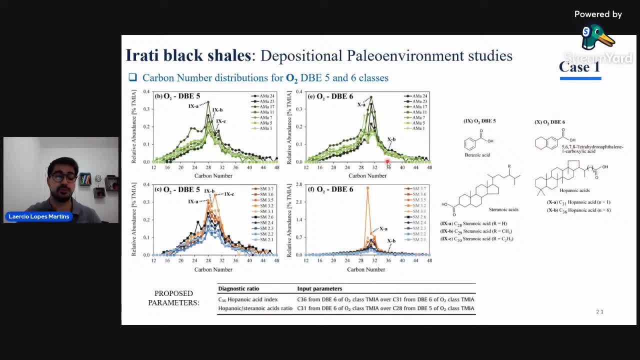 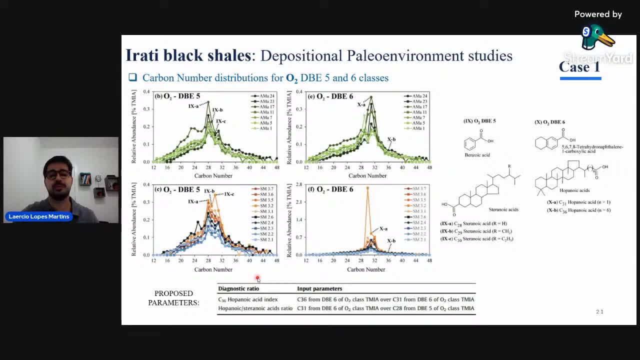 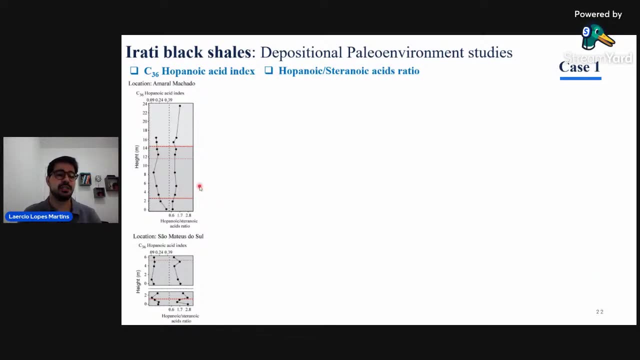 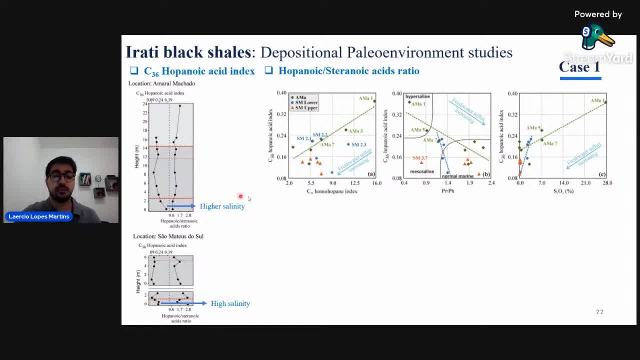 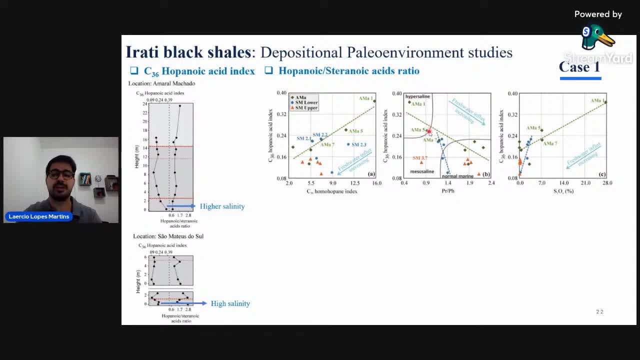 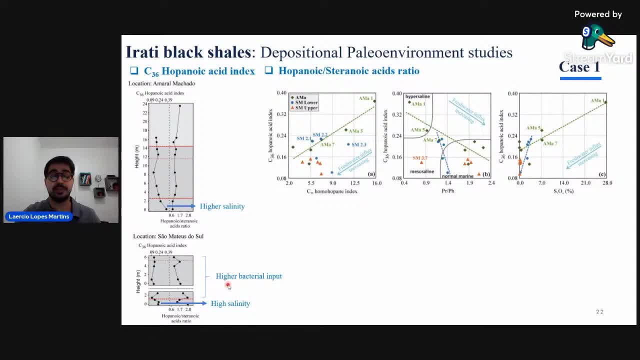 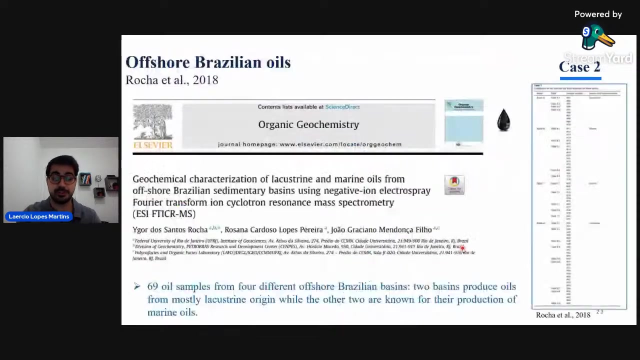 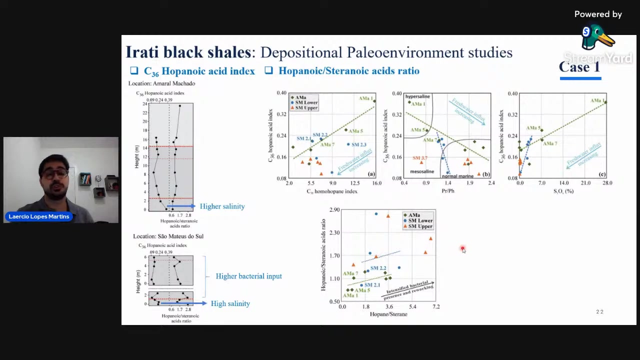 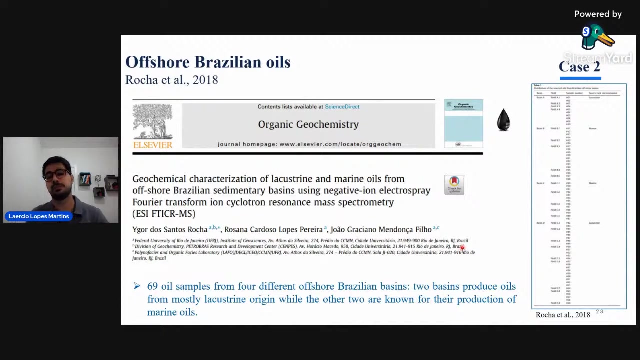 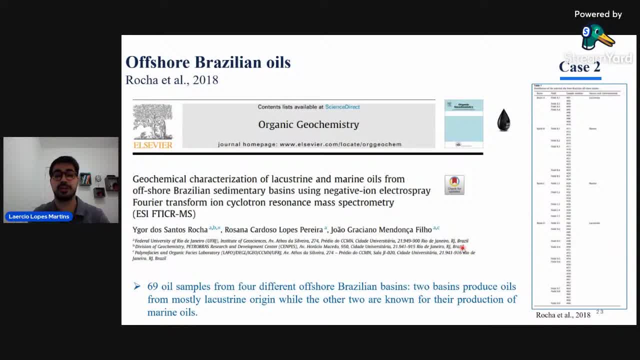 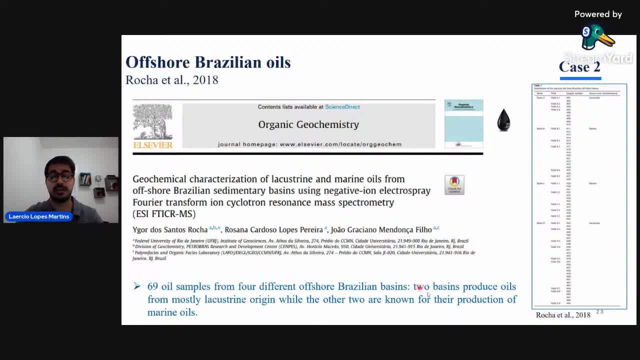 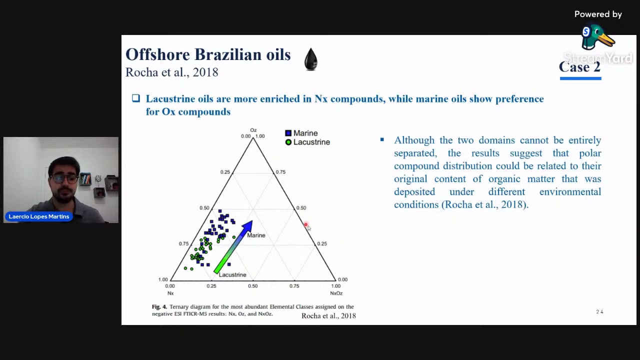 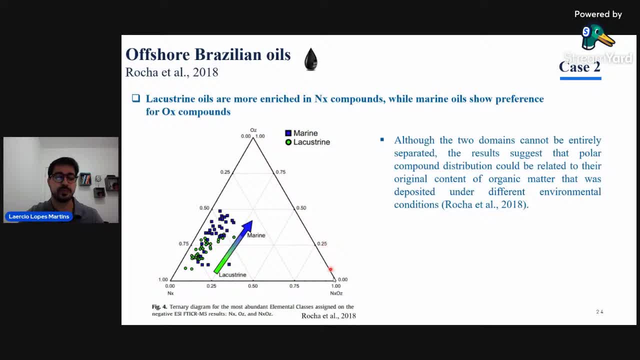 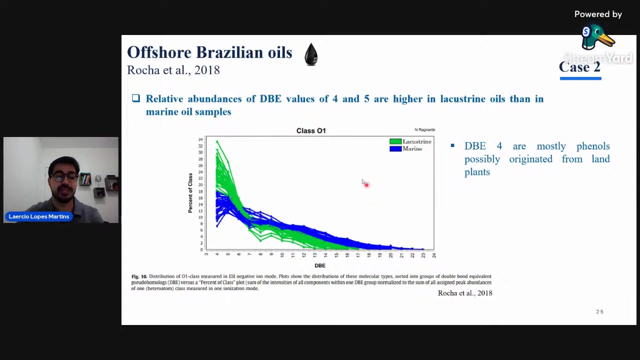 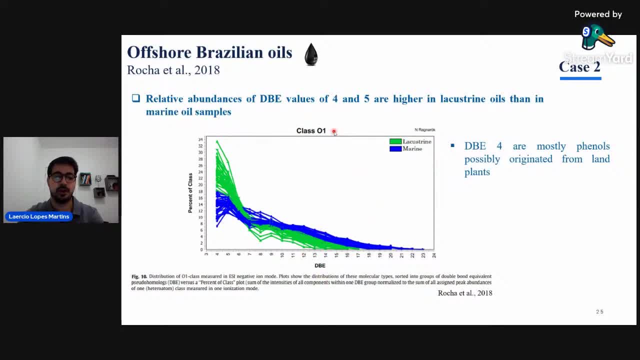 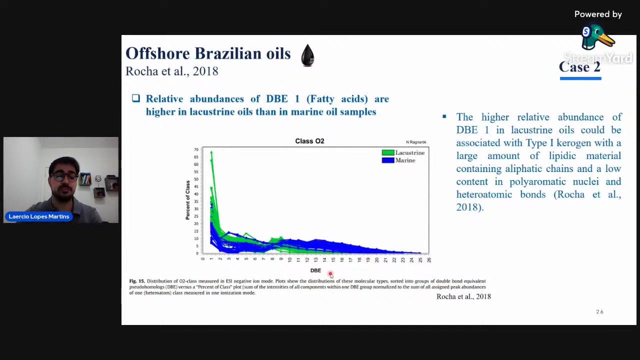 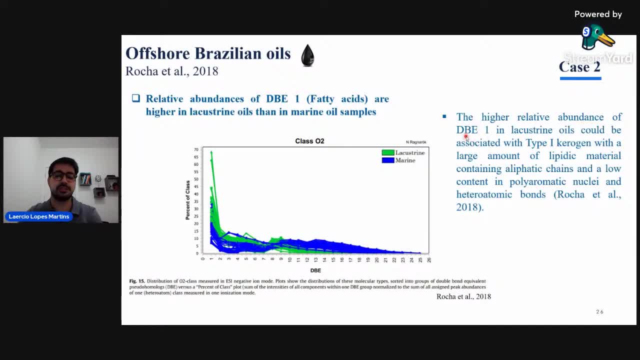 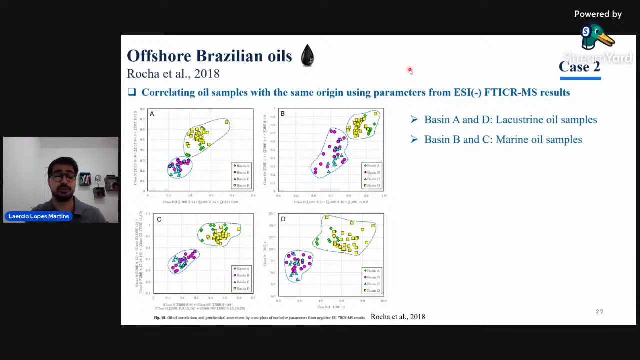 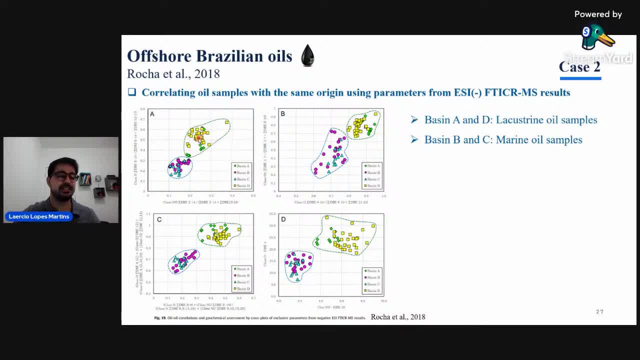 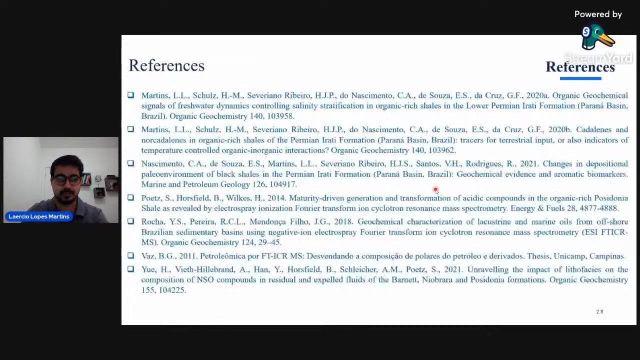 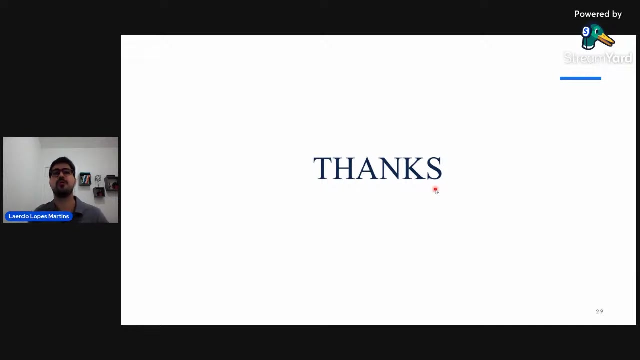 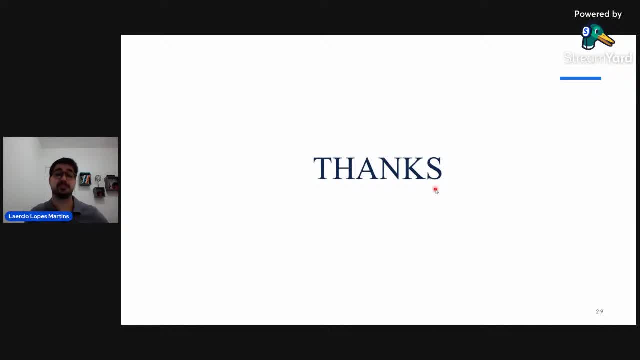 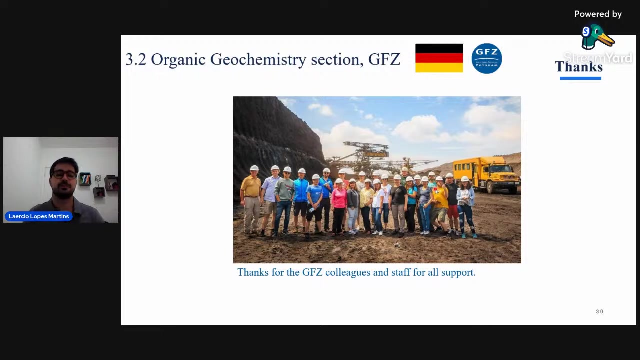 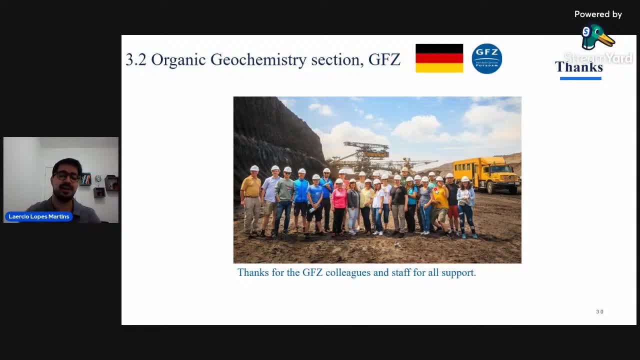 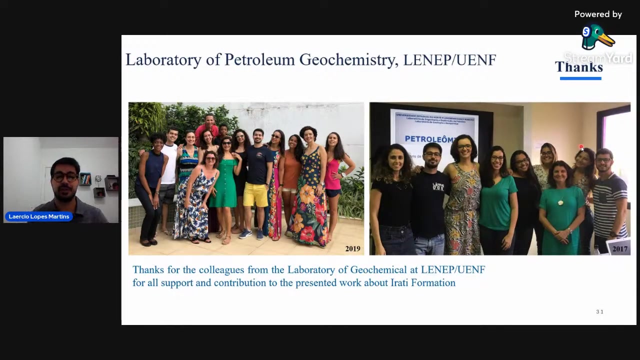 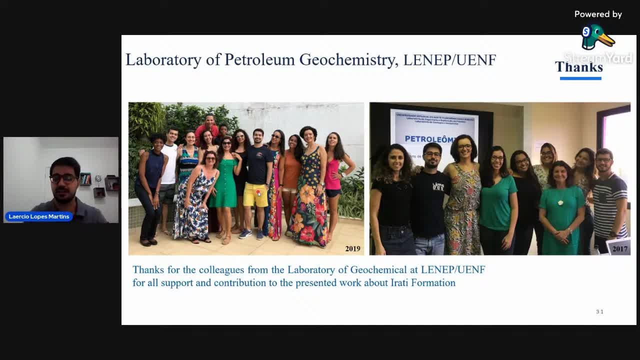 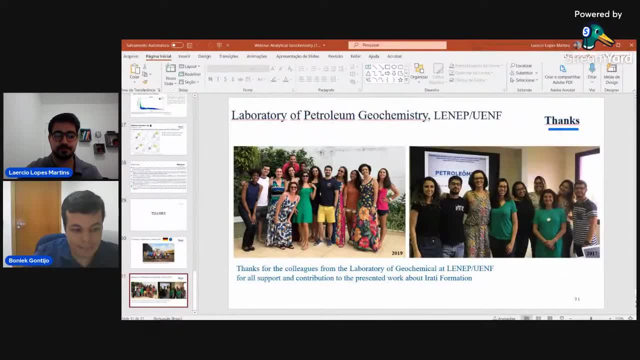 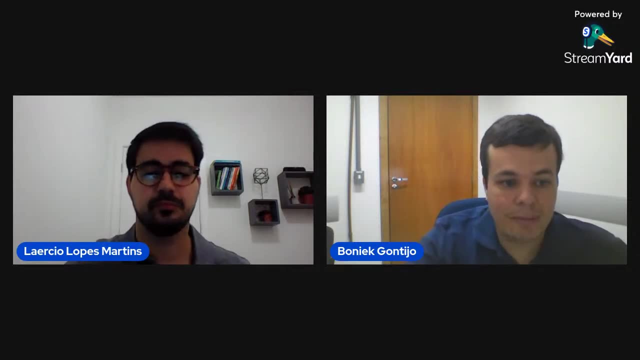 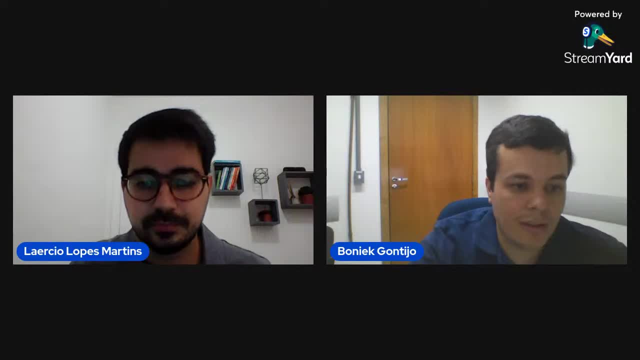 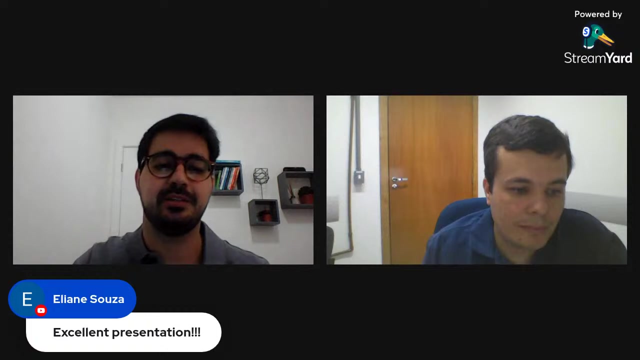 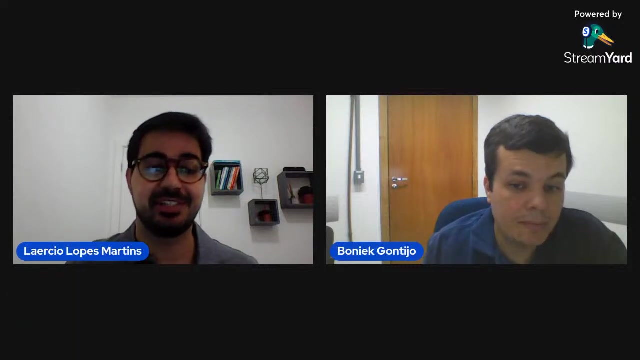 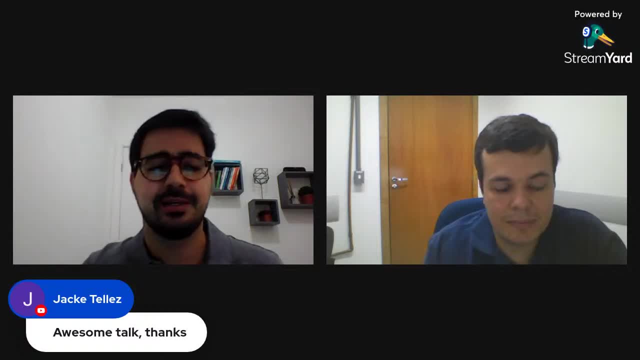 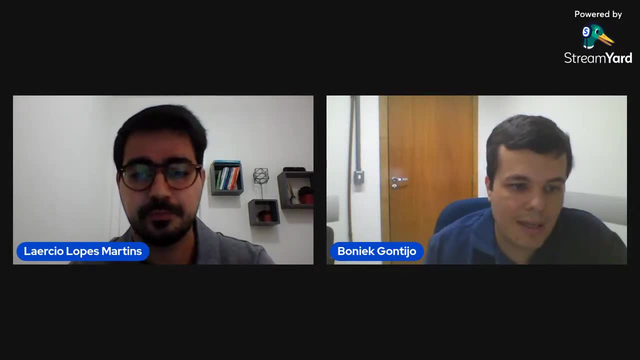 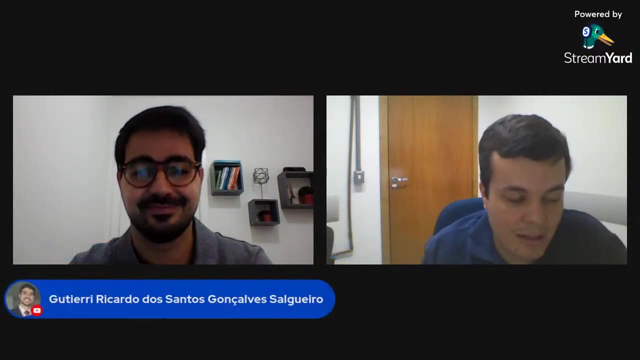 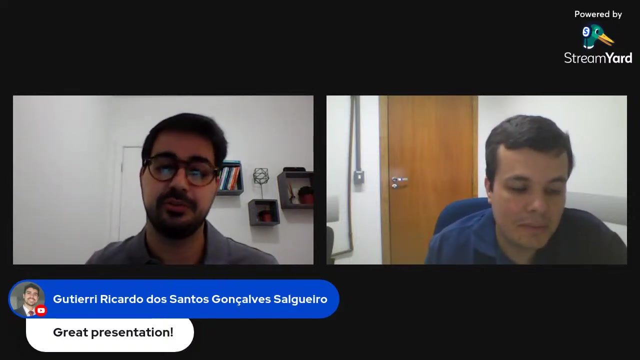 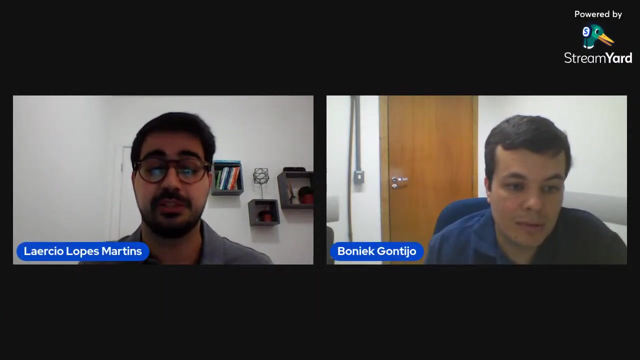 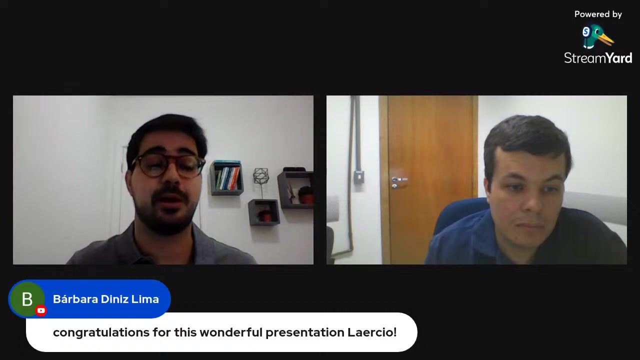 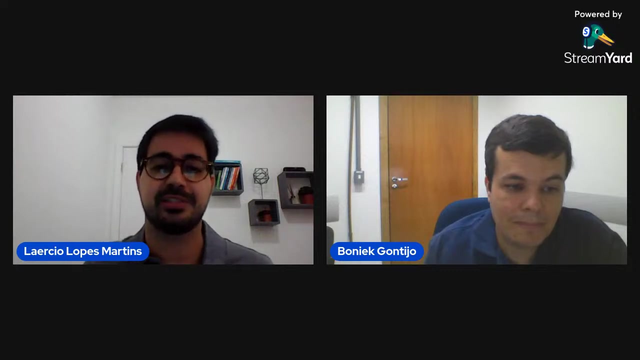 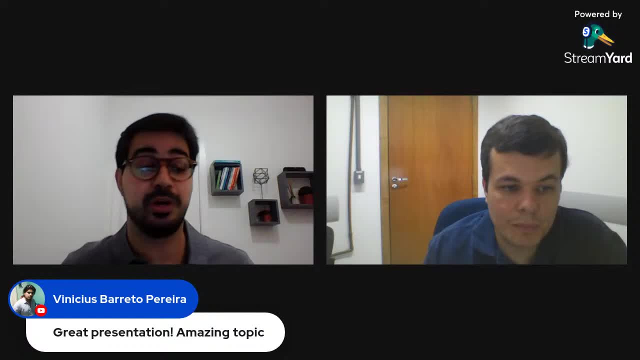 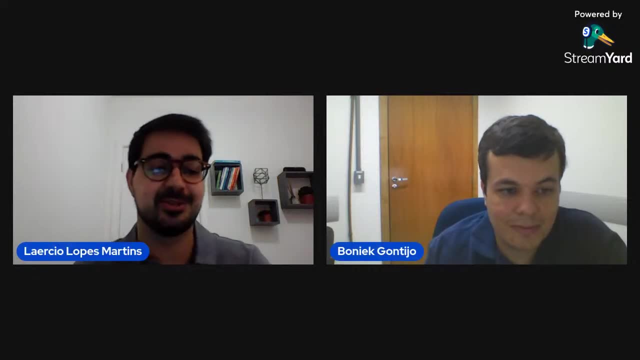 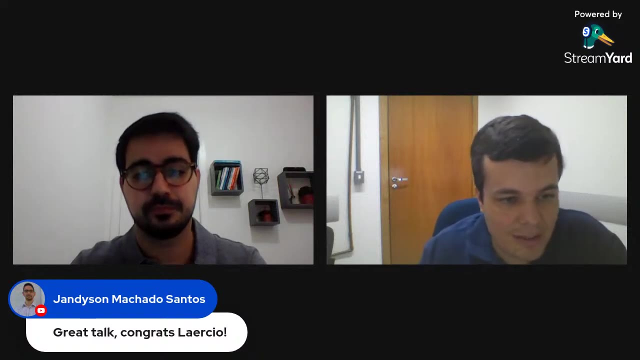 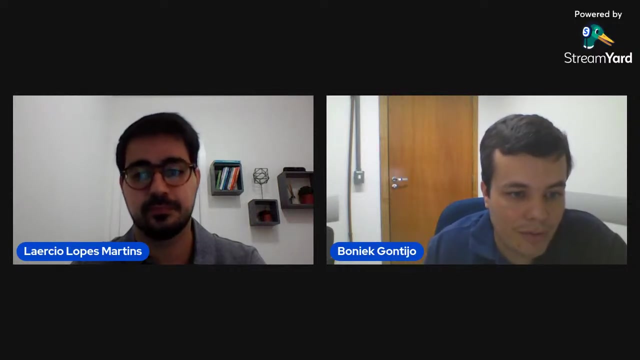 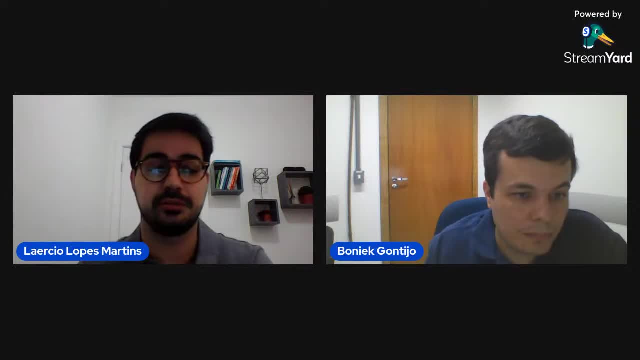 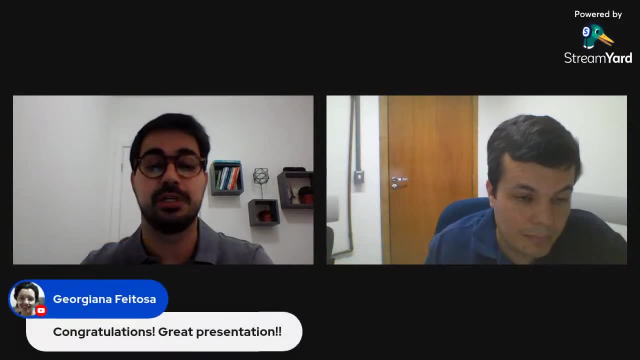 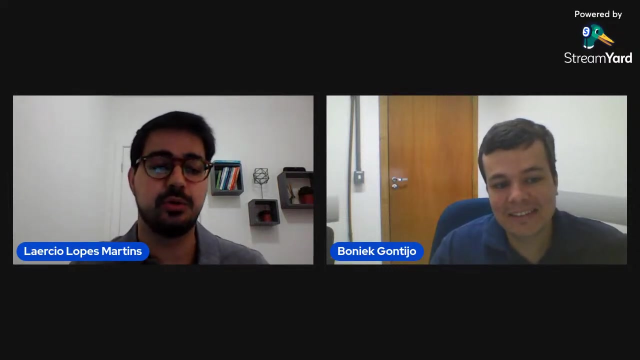 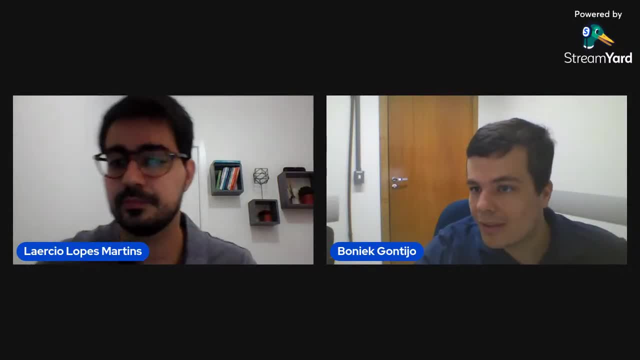 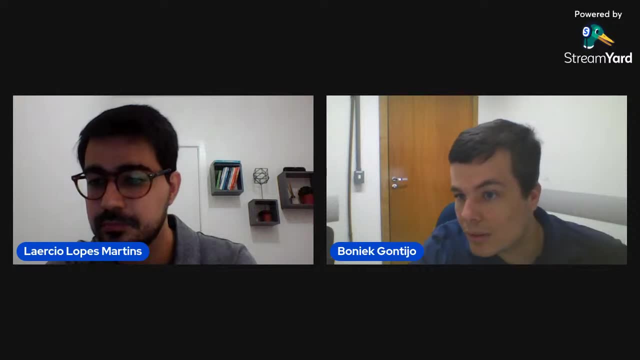 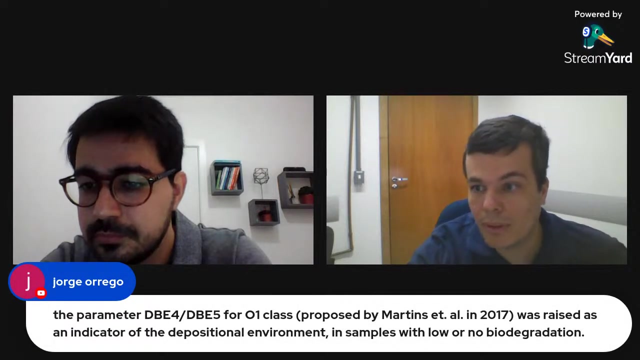 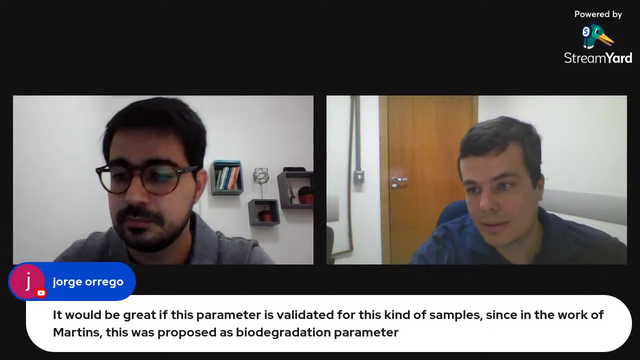 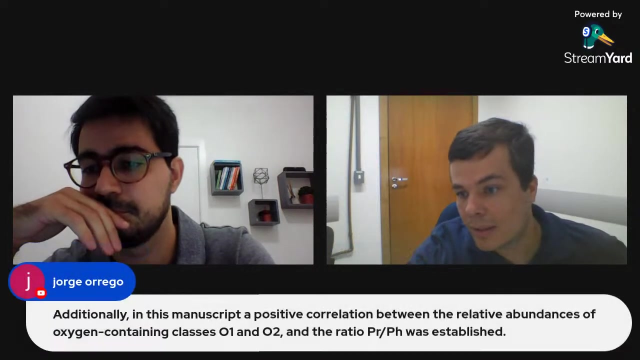 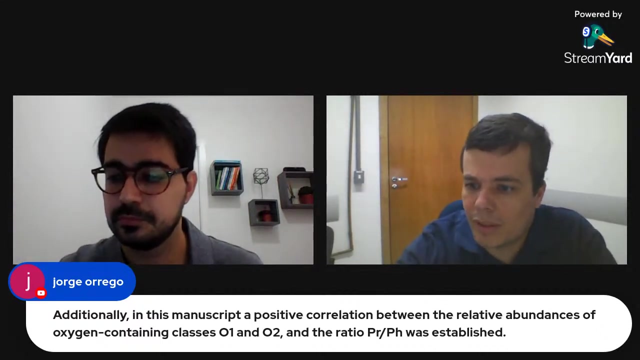 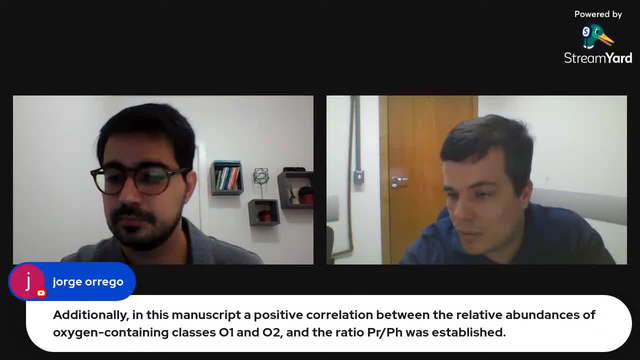 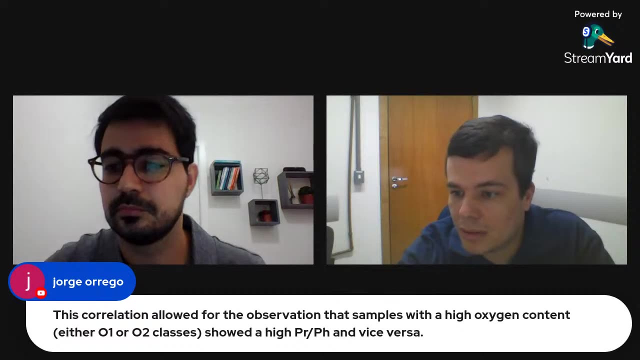 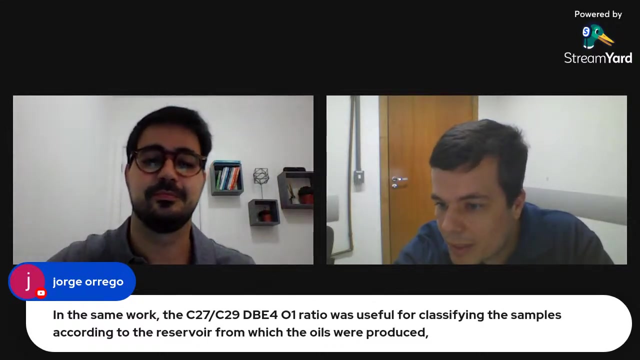 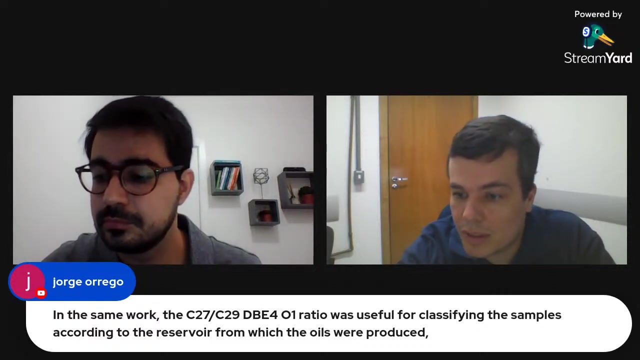 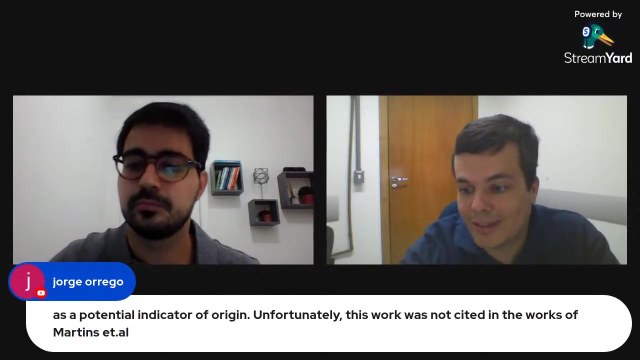 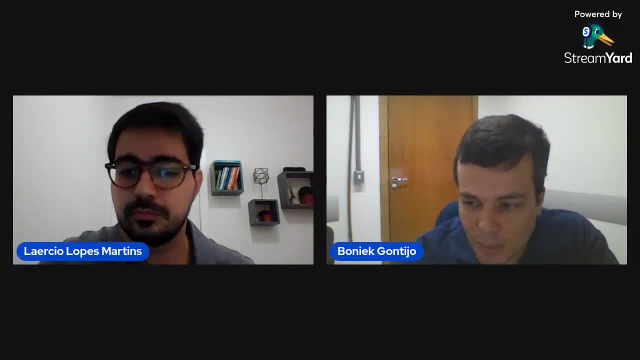 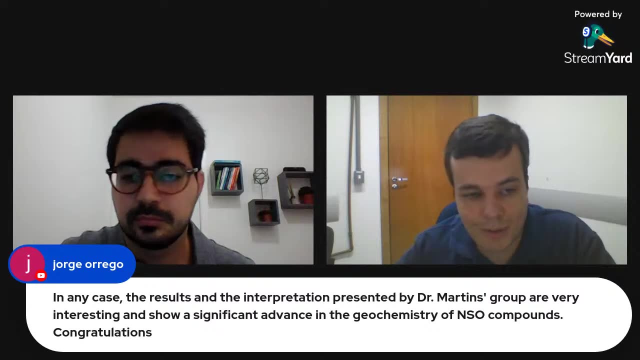 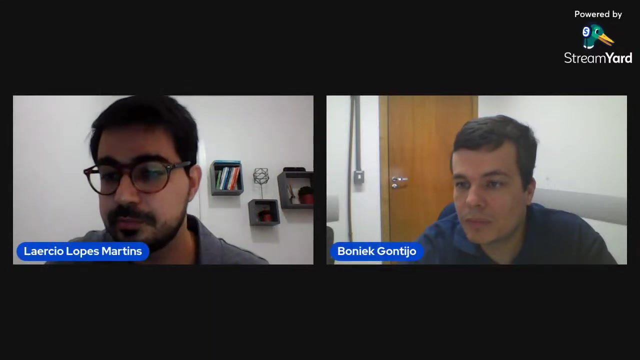 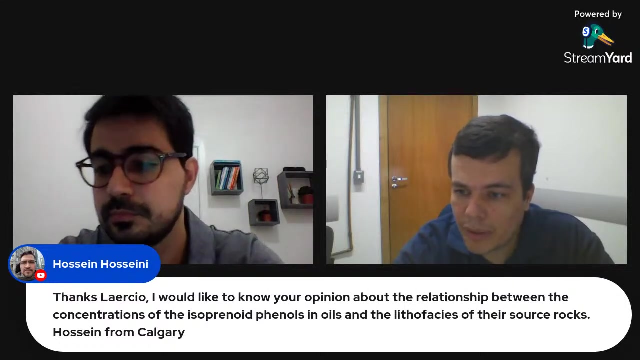 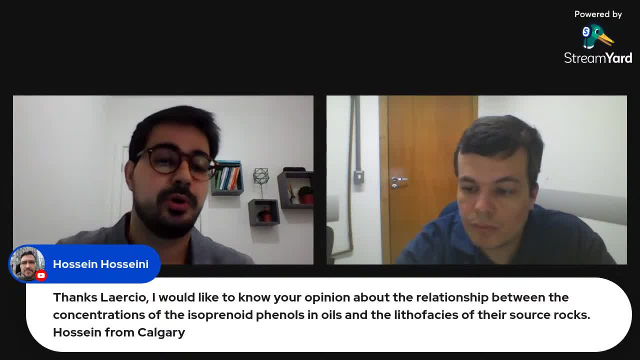 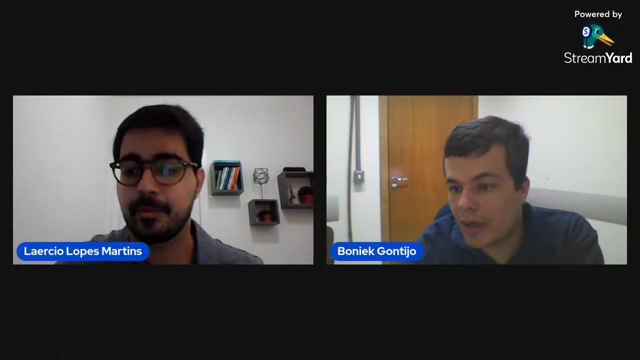 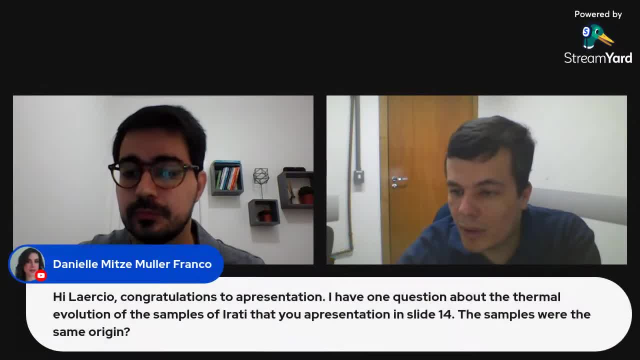 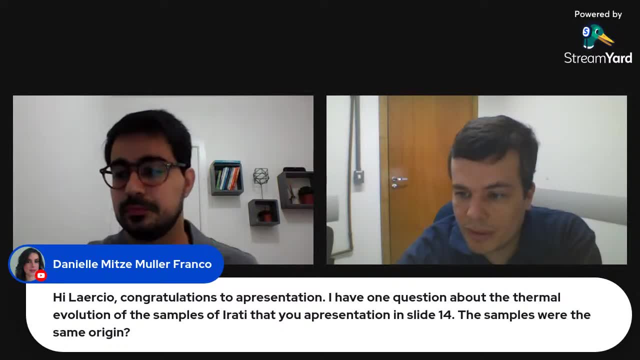 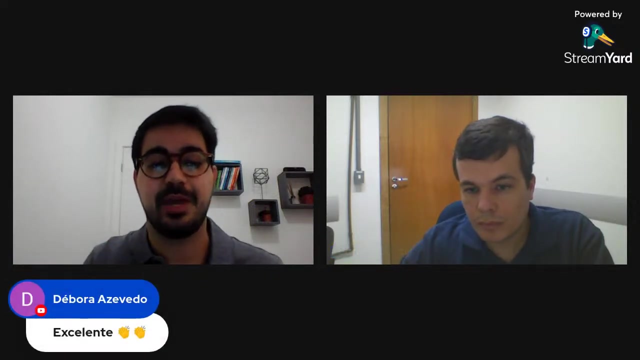 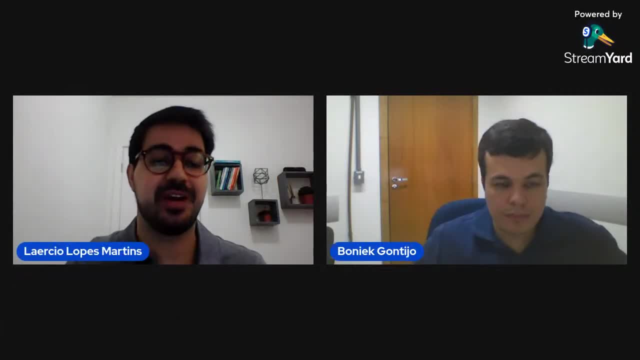 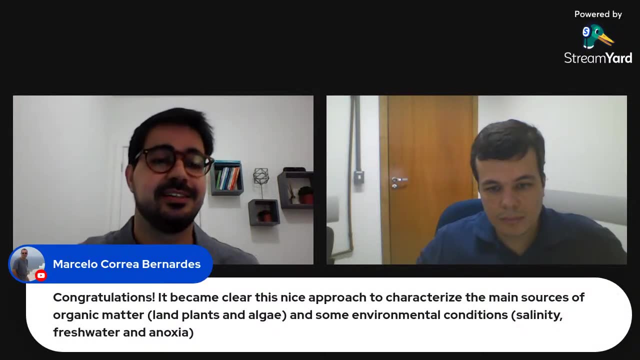 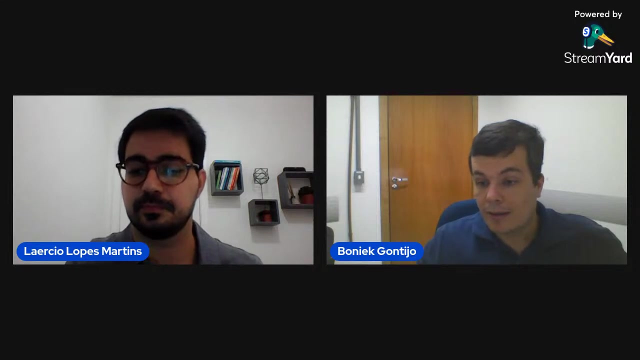 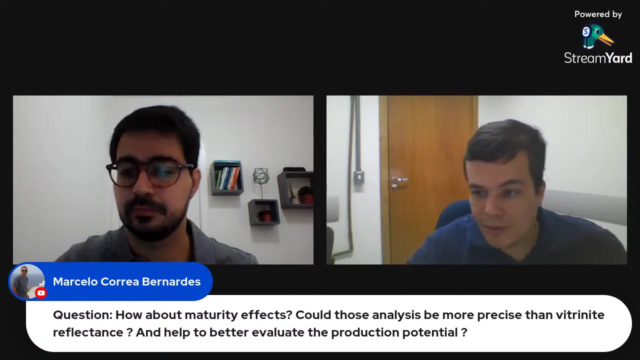 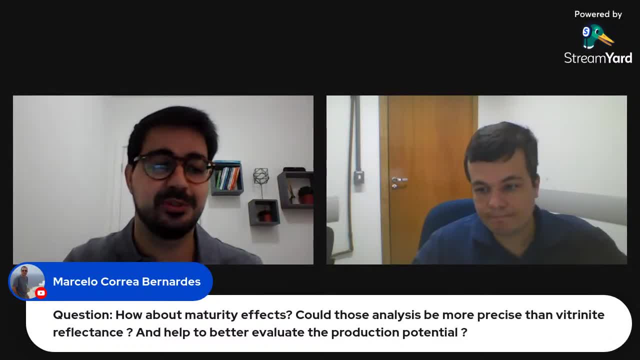 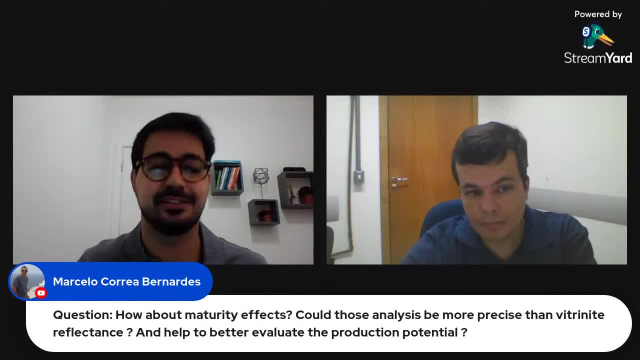 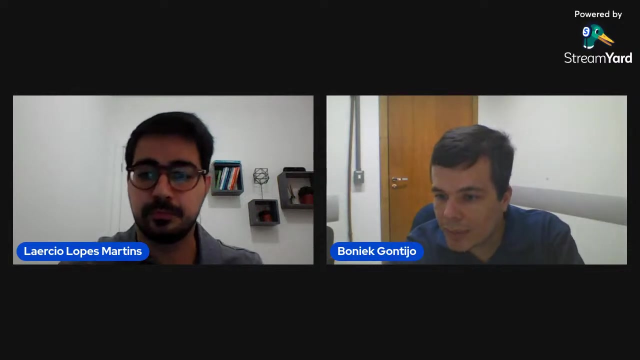 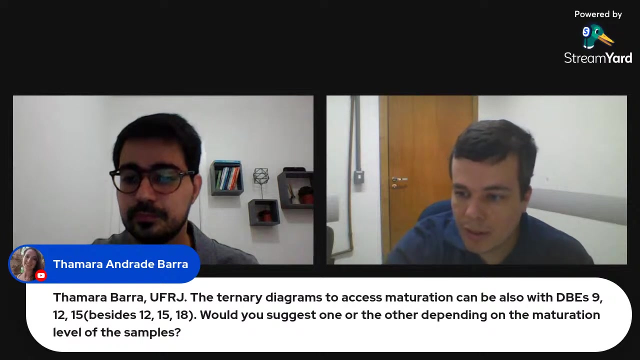 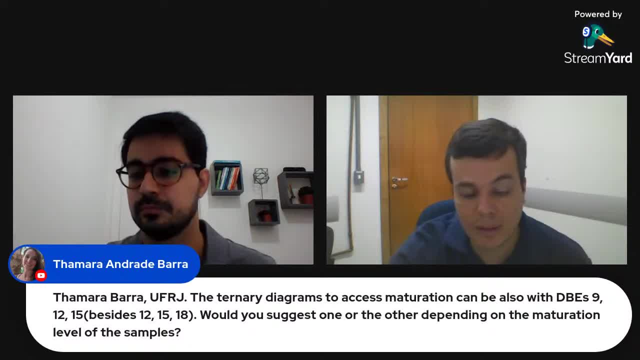 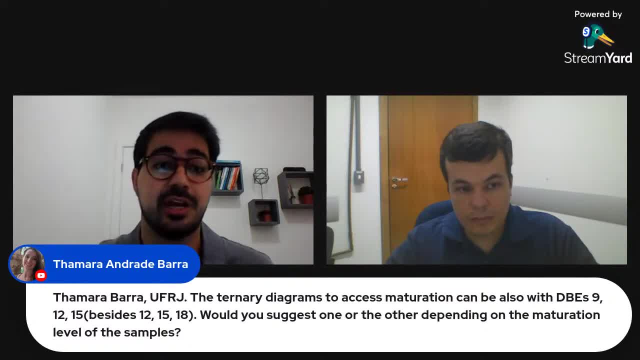 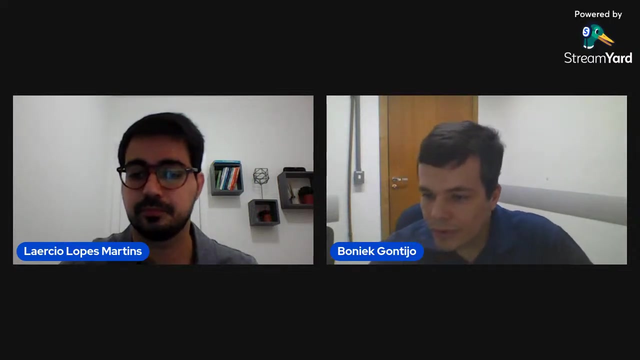 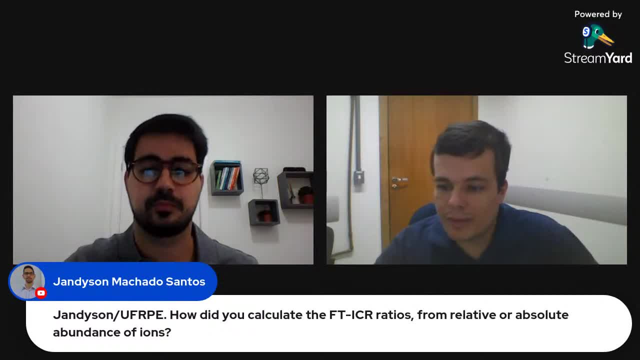 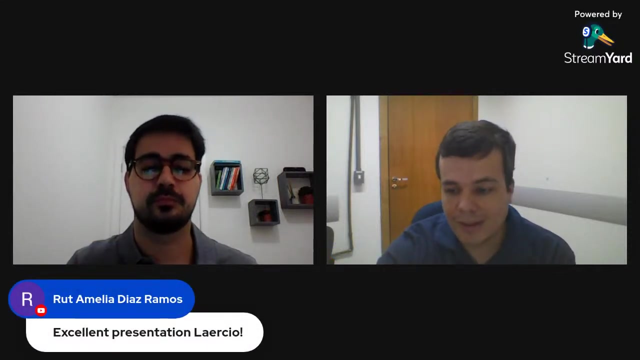 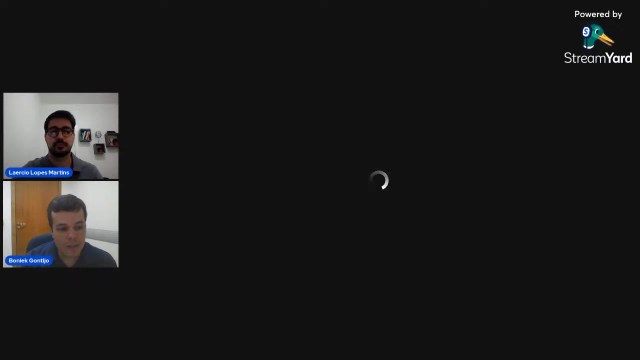 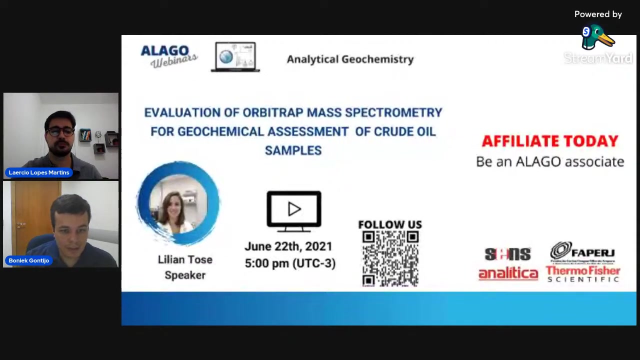